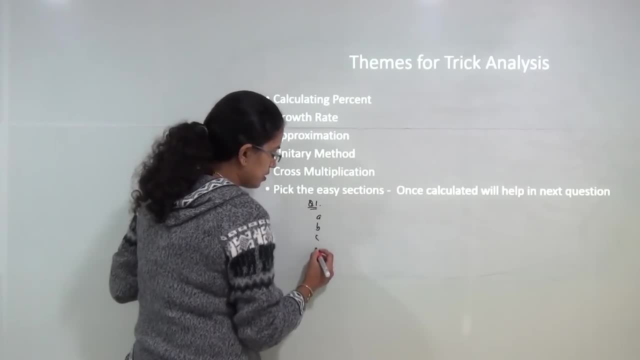 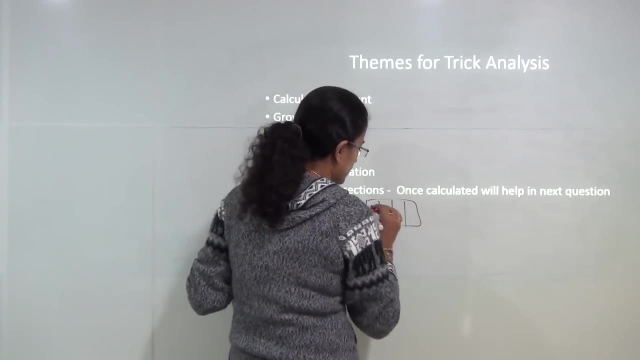 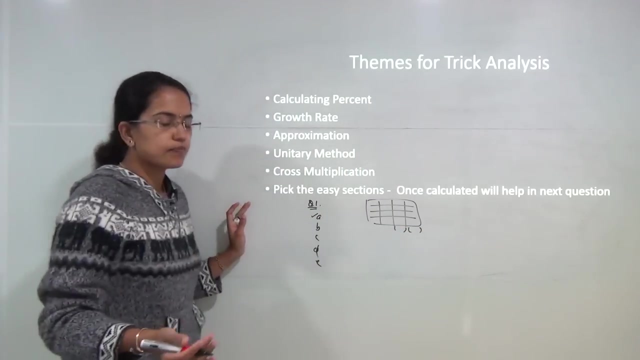 in the words e. view of one section. Many questions can be solved in a given question. On a question on data interpretation, usually you have 4 to 5 subsections that are asked. Now, when there is, say, let's say, table, and you have to calculate the totals for solving question A, so those totals would again be. 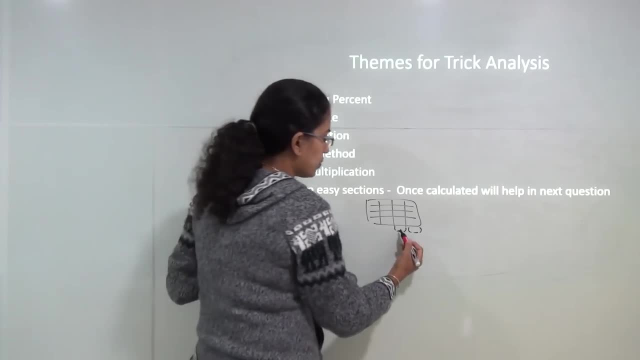 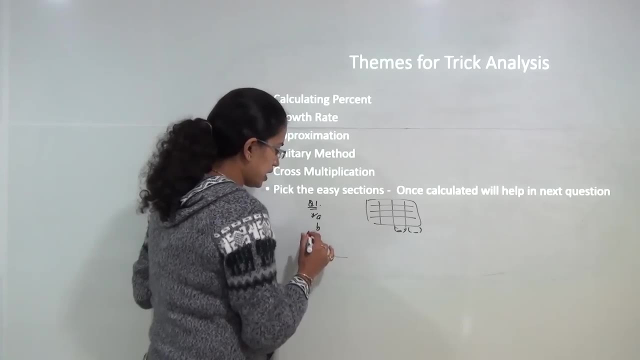 applied to question D and sometimes it is such that you have to calculate the totals and those would be have in question B, so it is okay to do in question A. Now房 question. question D would not be asked in question A, but some of it might be applicable in question. 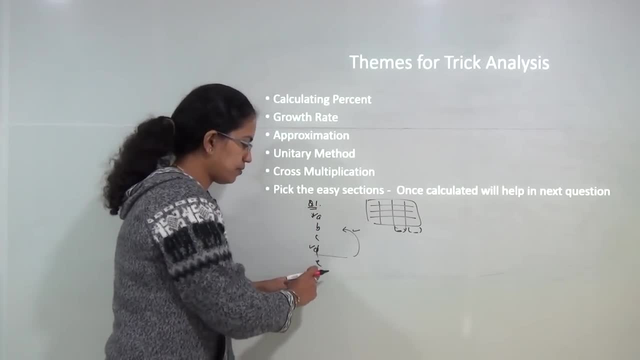 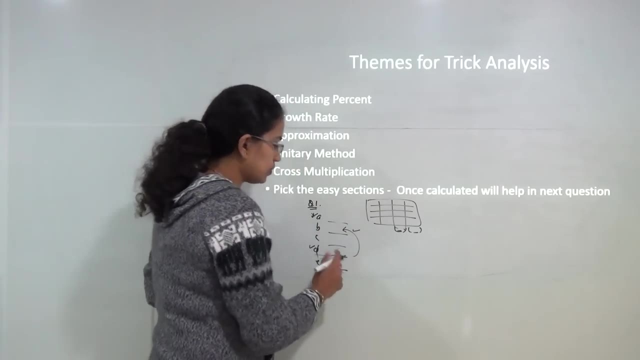 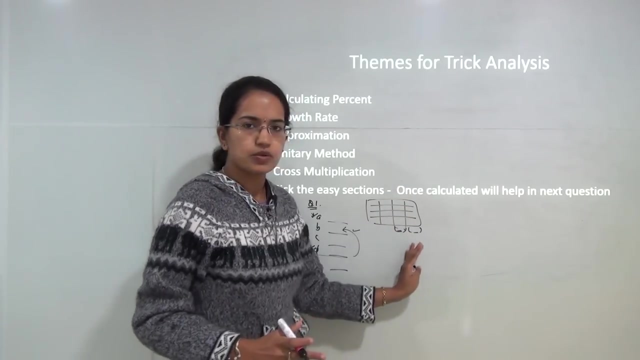 2. So that means if you are solving the questions in alphabetical order you might take a lot of time. So the best idea is to read all the questions at the first go and see what all kind of data is required. So if some of the questions required deriving it from the total start working with the totals. 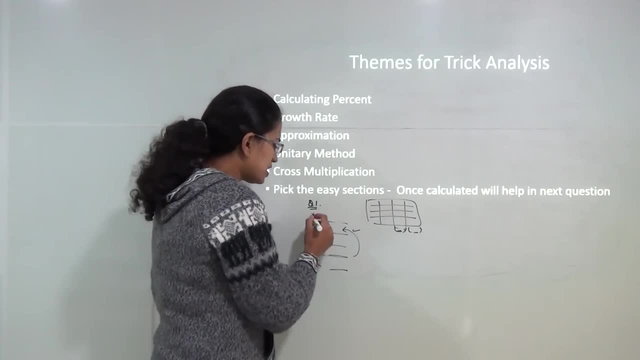 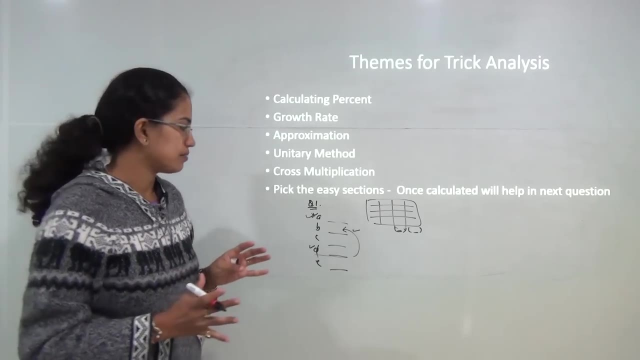 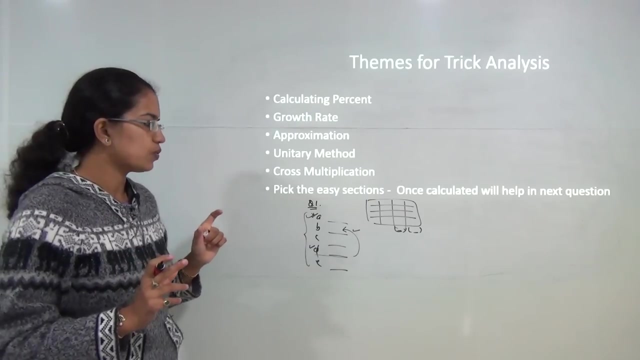 first and then proceed on. So these are some of the techniques that will save time in a exam where you are really running short of time. Also, of these 4 or 5 questions, there would be just 1 or 2 question that would require. 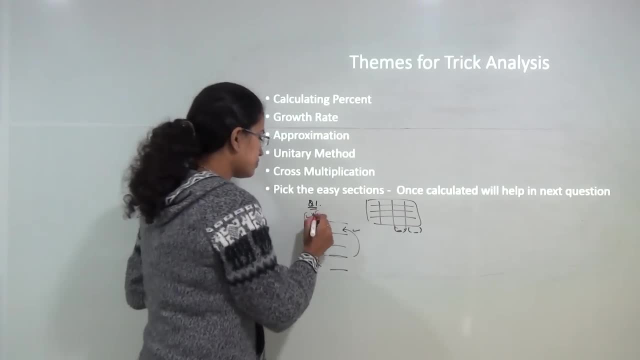 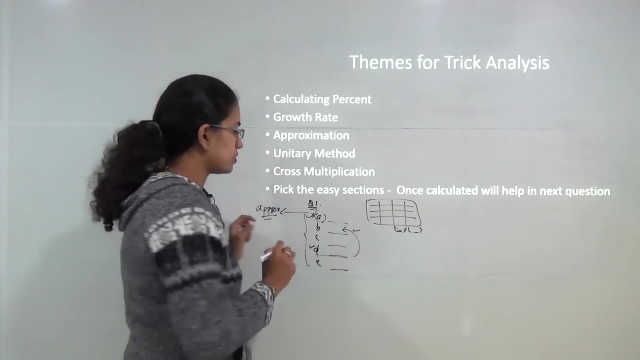 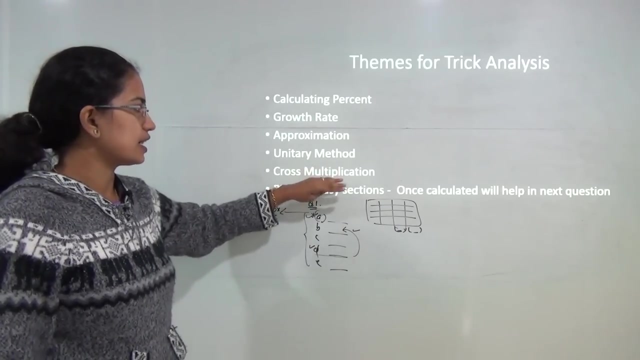 really time consuming calculation. So you can either leave those towards the end or you could apply techniques for approximation that we will discuss further in this video to work around quickly for solving such questions. Okay Now, the first thing that we will understand in this class is approximation. 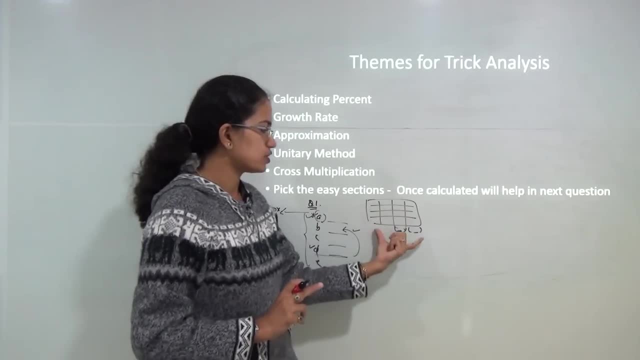 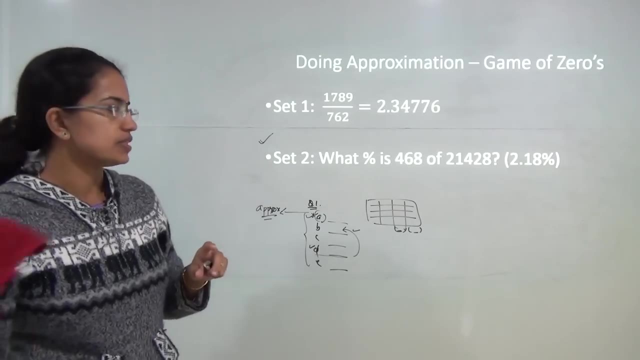 Now, this is the key aspect for most of the questions that are asked based on tables, and the questions that require lengthy calculation. So most of the students are struck up when it comes to approximation. We will learn some quick tricks on to how to solve the questions of approximation. 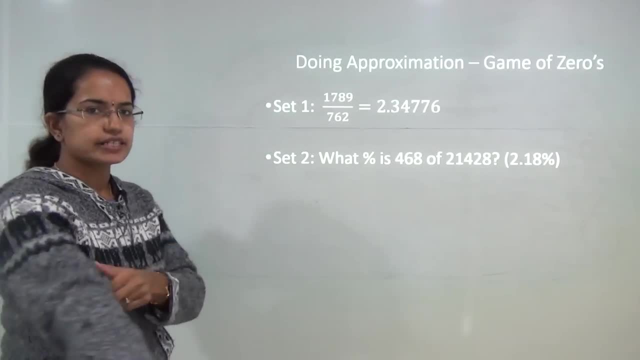 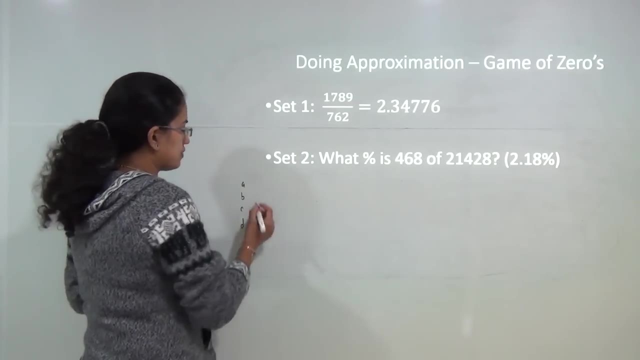 Now, when there is a question of approximation, the first thing that is important is to look at the choices. If the choices are really far away, Say, for example: if the choices are really far away, Say, for example, question 1, if the choices are 2,, 5,, 6, or say 1.. 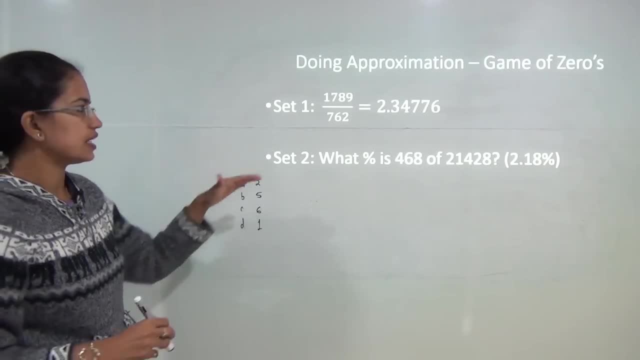 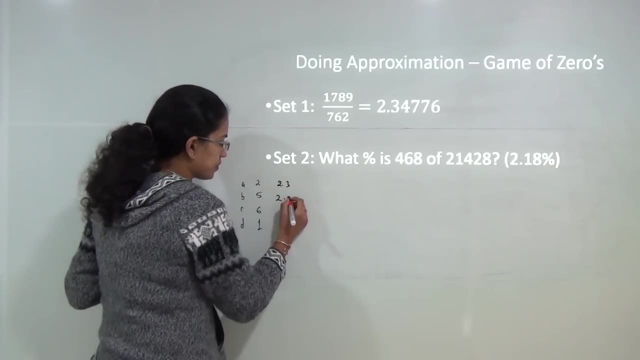 That means the choices are really far off and you can easily say what would be the answer. However, if the choices are close- by say 2.5, 2.3,, 2.5, 2.8 and 2.9- what we will do 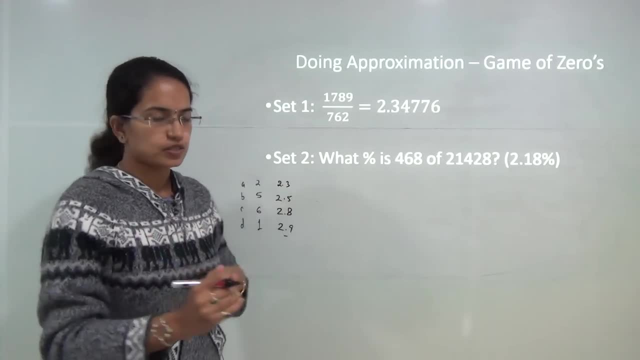 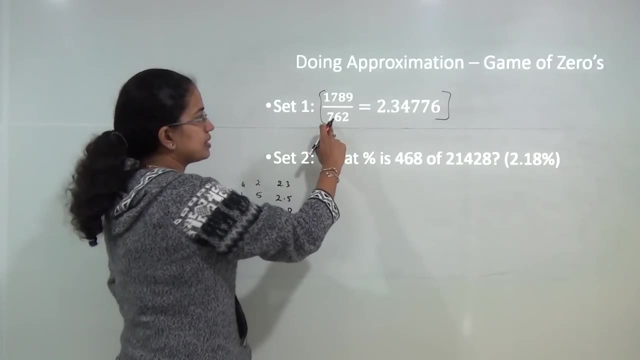 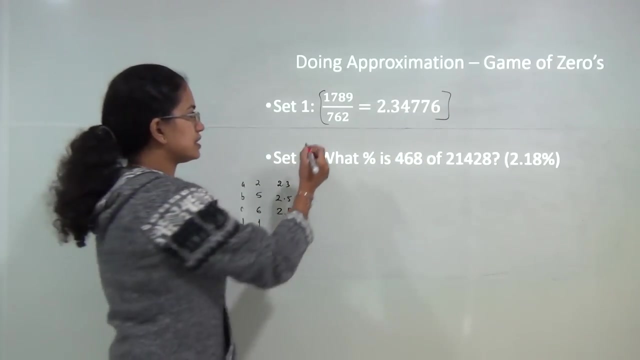 Then you will need to apply bit more of approximations. Now, how to work around a question like this? You have 1789 divided by 762 and the exact answer we know is this: Now, when we apply the technique for approximation, let's say, I approximate this value to 750.. 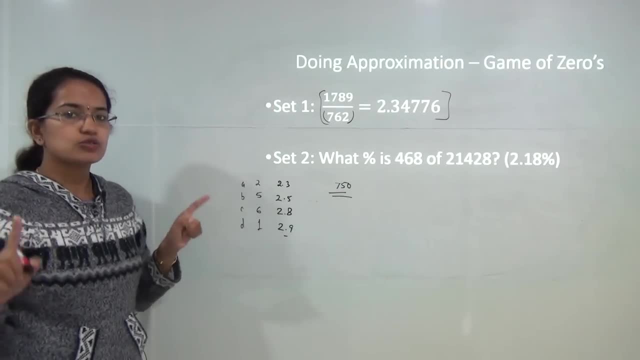 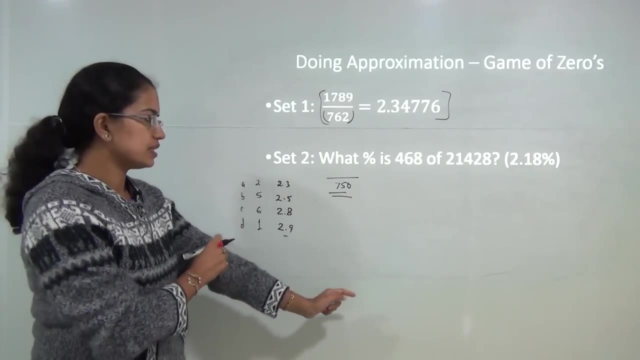 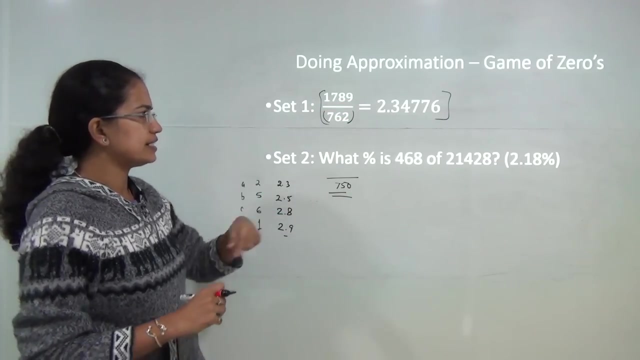 Now the main idea is to approximate the values close to 0. So once you have 0 in the denominator and the numerator, it would be easier to solve. So, for example, If I reduce 12 here, That makes it 750, and on the top side let's- by visualizing this, I can say it's more than. 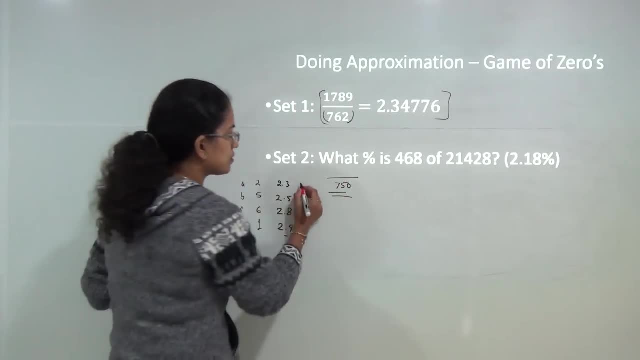 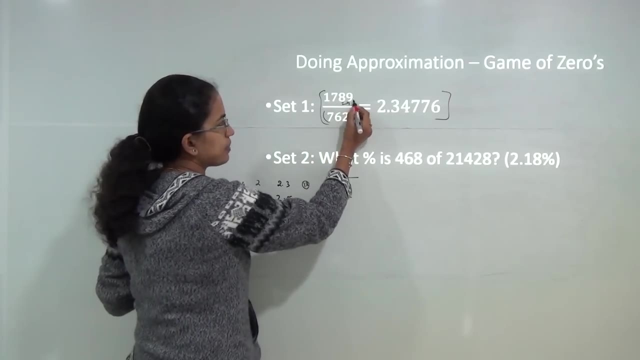 double. So I will do more than double. So I am reducing 12 here. So double of 12 is 24.. So I will do more than 24.. So let's take a number which makes the last figure 0. So then I can say 29 would be the appropriate number. 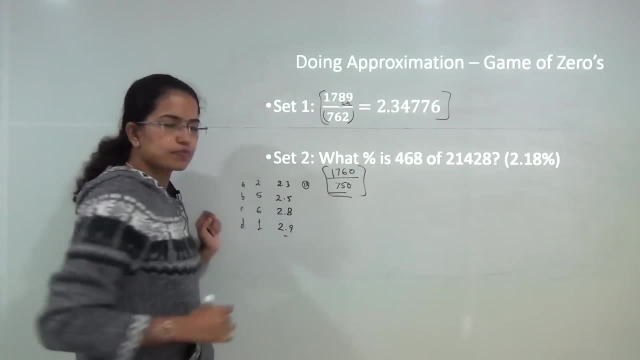 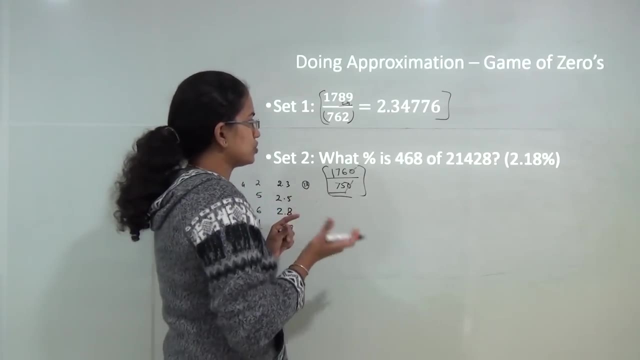 So I can say 1760.. So this is one way of approximating. Then I can cancel out the 0s and solve it. So that's it, Thank you, In a much quicker way. Another technique that I usually work around is you take 750. 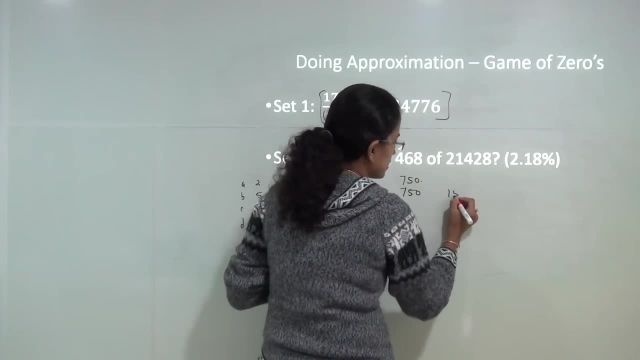 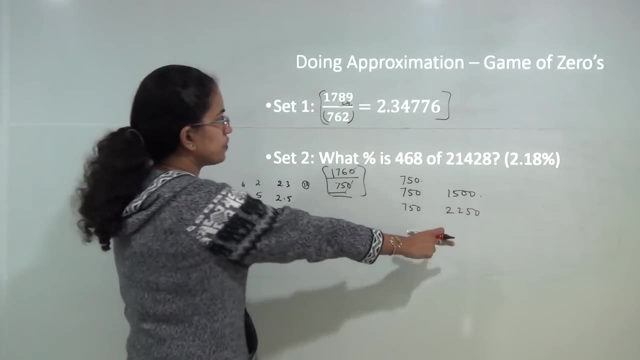 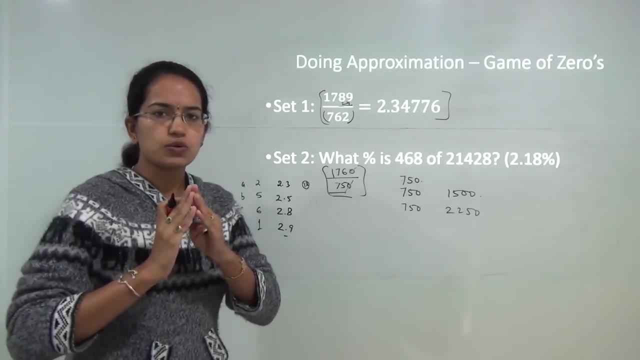 Then another 750 will make 1500. Then if I do another 750, that will make it 2250.. That is too far away from 1789.. So what I need to do is let's break this 750 into 3 parts. 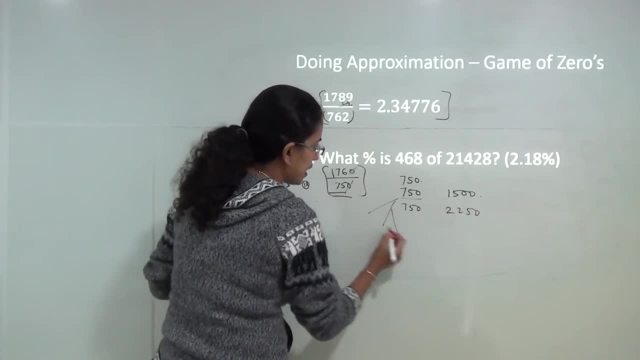 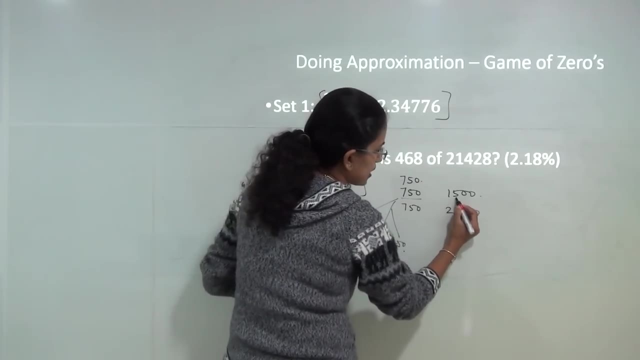 So if I break this 750 into 3 parts, Let's see what we can solve. So we will do this. start with taking the 8. gave the 8. three parts, I can get 250, 250 and 250. now let's simply add 250, so 1500. I add 250. that 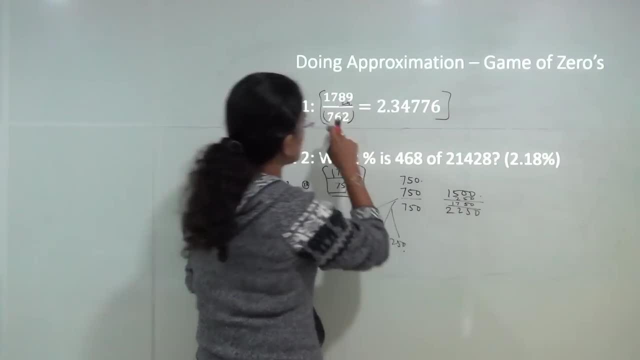 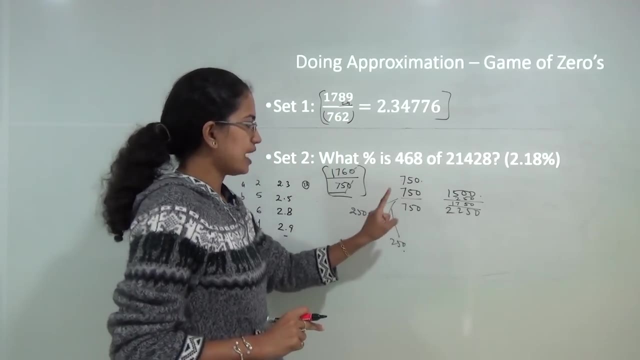 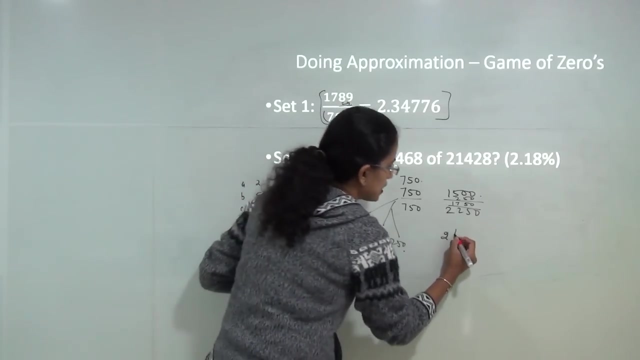 makes it 1750 and that is very close to 1789. and this 250 is one third of 750. that means I am using 2 times 750, that is 2 and one third of 750, that is 2, one third. or I can also write: 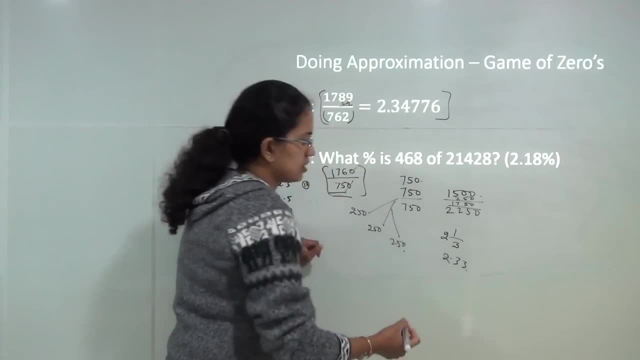 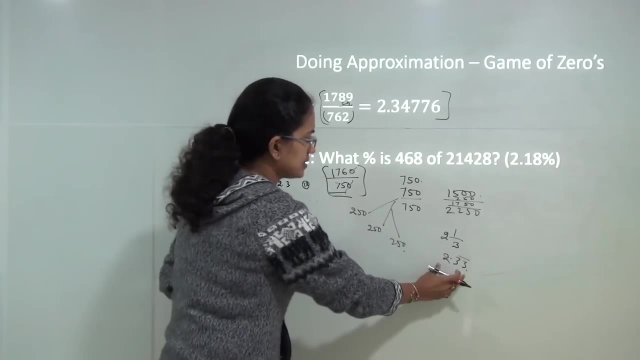 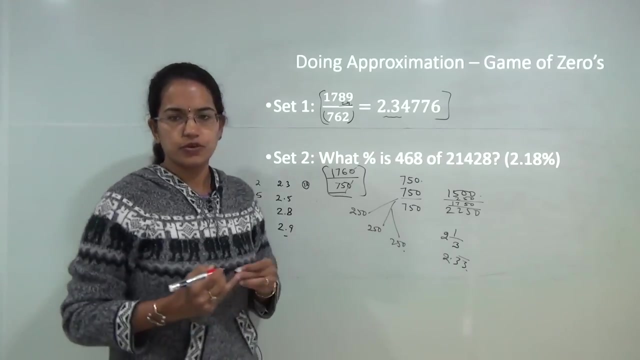 it as 2.33 and I can put a bar that says it is a recurring decimal, however. so my answer, I can say, would be close to 2.3 and if I look at exactly, the answer comes to be 2.34. so that means this is one of the techniques that you can use to calculate the number of parts. 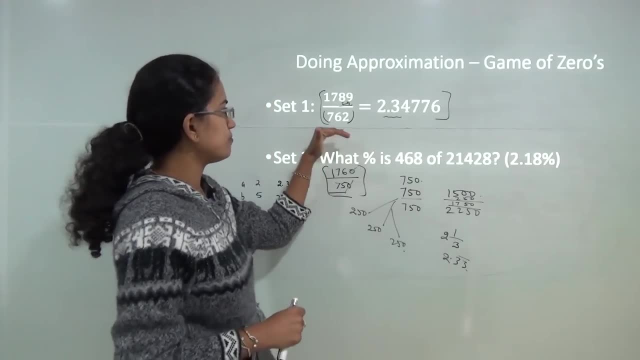 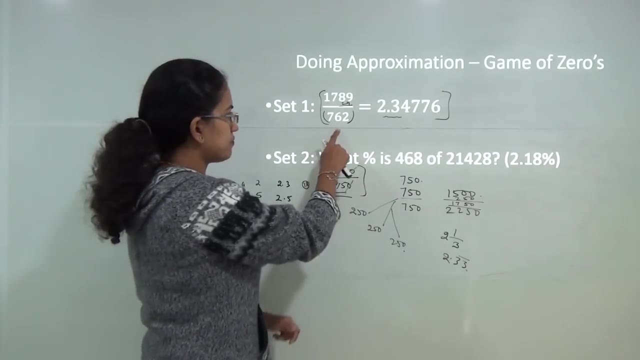 that you want to add. So the next method that you can apply for approximation- I repeat again, what you can do here is there are 2 ways in which I am explaining this approximation method. the first is you do 750, you reduce 12 and then by visualization you can see it is nearly. 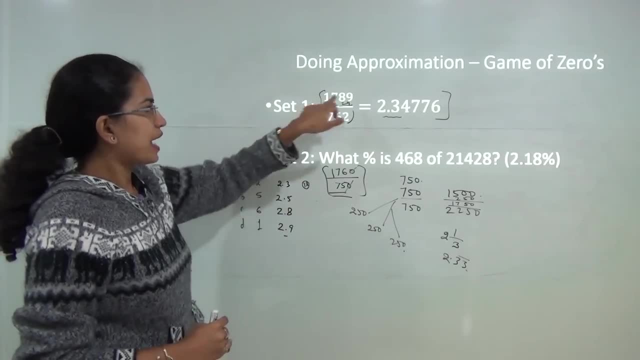 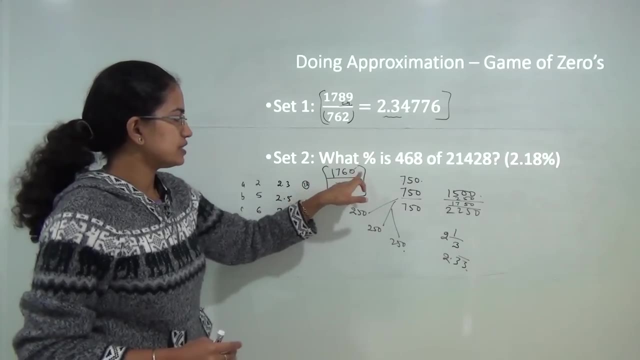 double of it. so you double 12, that is 24, and then, since last digit is 9, I make it 29, so as to make the last digit 0. so it becomes 1760 divided by 750. I can cancel out the 0s. 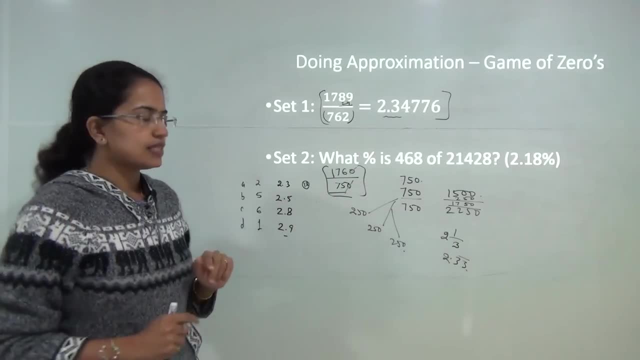 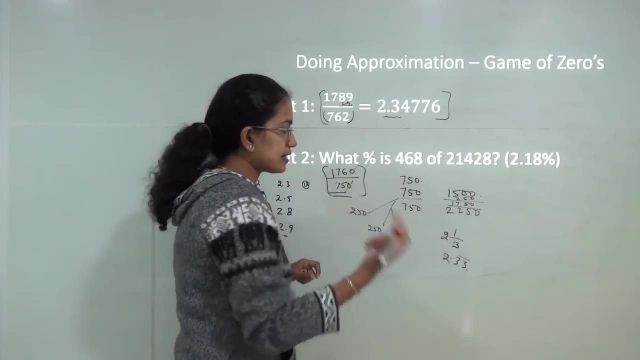 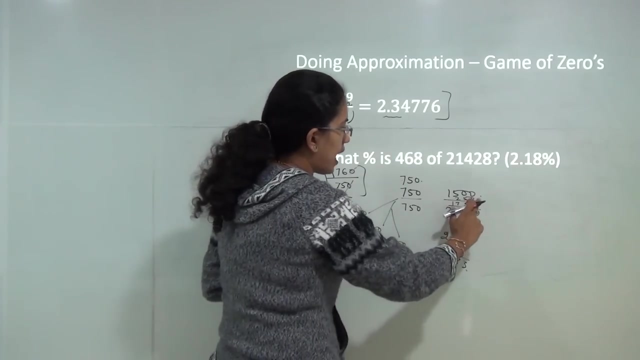 I can simplify this fraction to work around. that is one method. the another method is: I add 750 and 750. that gives me 1500. now if I add another 750, it gives me 2250, which is very far from the given numerator. so what I do is I divide this 750 into 3, equal half. 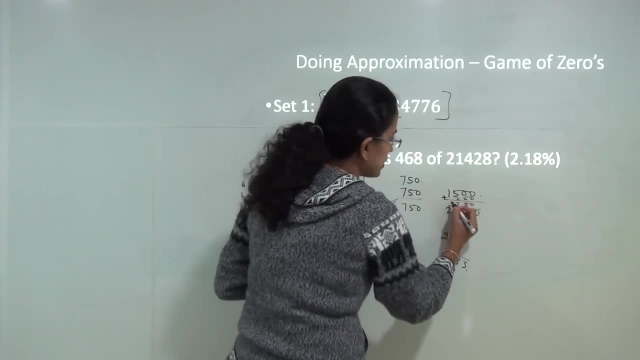 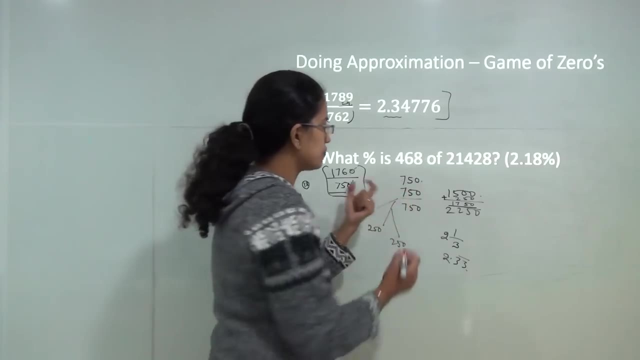 that is 250 each and I add 1250 to it. that makes it 1750. now this 1750 is very close to the numerator. That means my answer would be 2 times 750, so 2 and then one third times of 750. that. 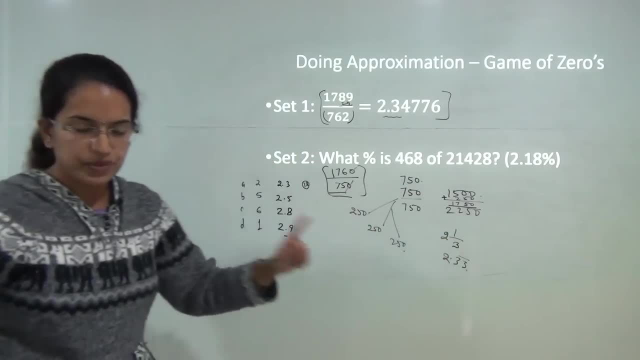 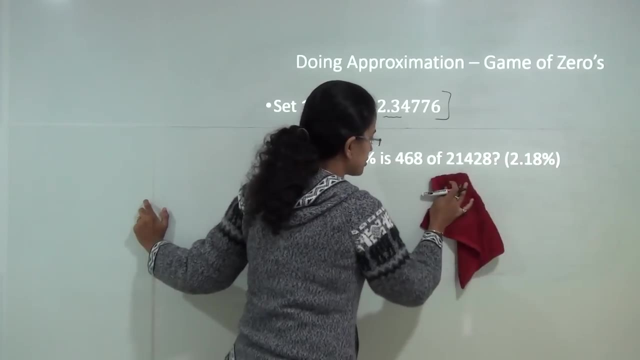 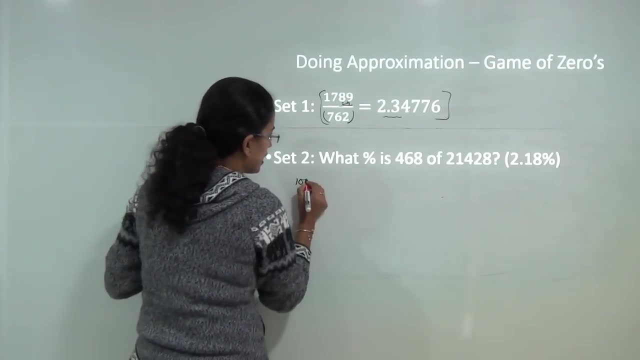 is 2, one third, that is nearly 2.33. so that is the first thing. now in the second set, what you have is: what is the percentage of 26? sorry, 468 of 21428. now, if I simply say 100 percent makes 21428. so, as you can see in most of the questions, what I am pressing is: I am pressing. 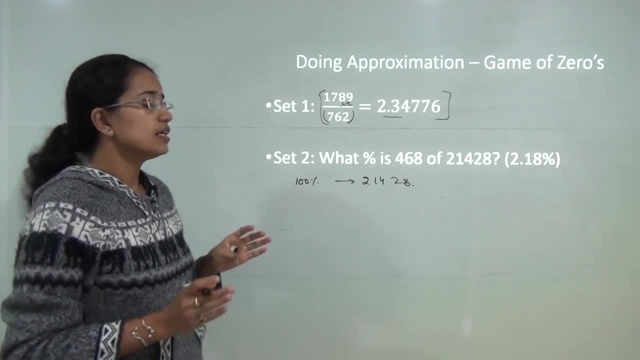 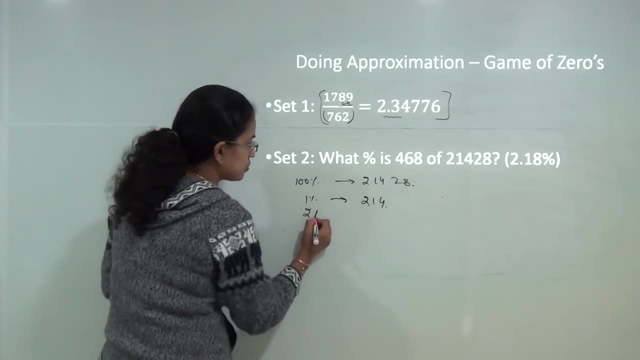 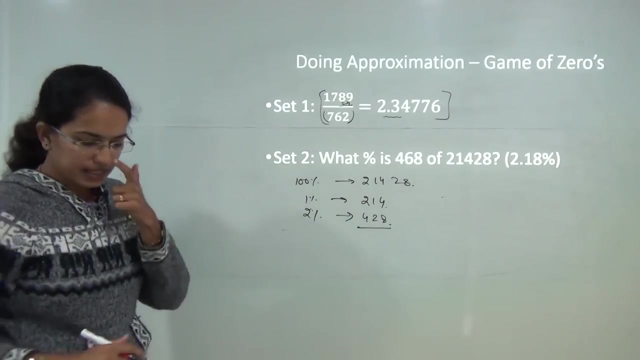 is applying unitary method, so that is the easiest way and the fastest way to work around. so 1 percent would be nearly 214. so I can say 2 percent would be nearly 428, and now this is 468. now if I do 3 percent, what it would be, it would become 3 times of 214, that is. 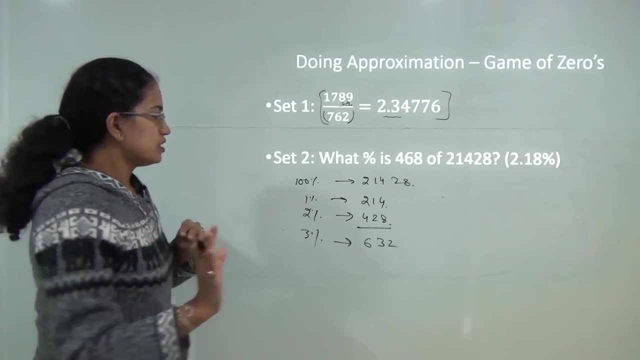 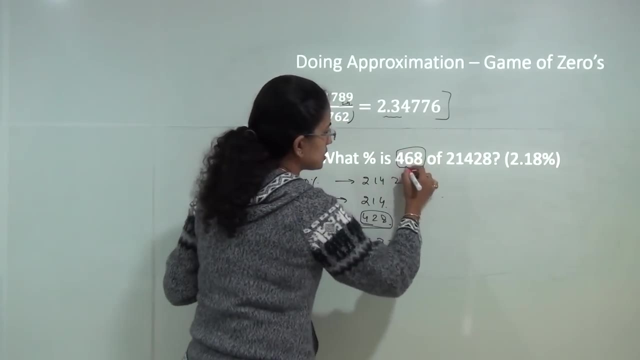 632. that is too far away. now my answer is: I already have 428.. So I have 428.. So I have 428.. So I have 428.. And my answer is 468. so my answer would be closer to 2 rather than closer to 3. now let's. 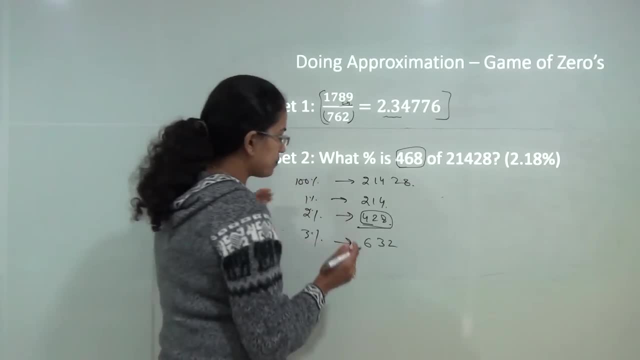 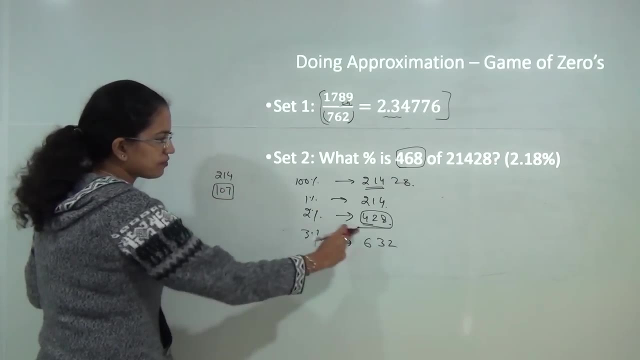 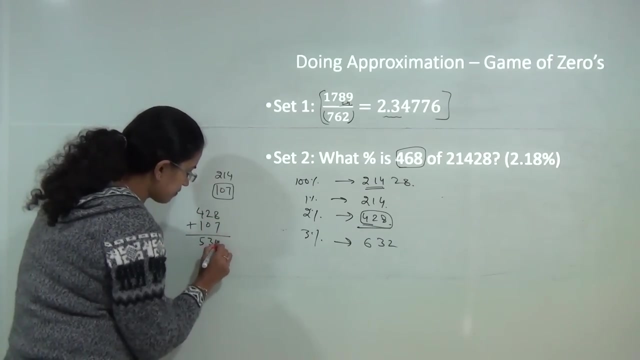 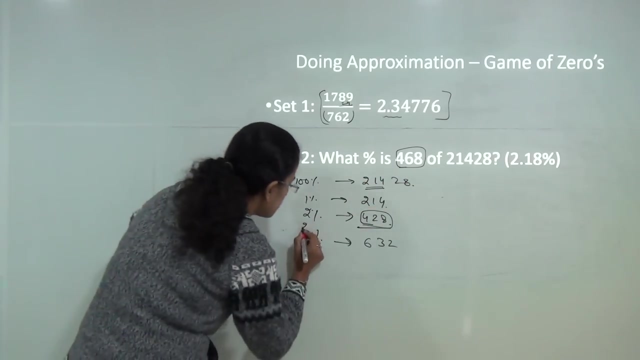 do a half way of it. so when I say half way of it, that means half of 214 would be 107. now if I had 107 to 428, that gives me 535 again. this is too far from the value that we need to derive. that means, if I take 2.5 percent- that also is very far from my answer- that I 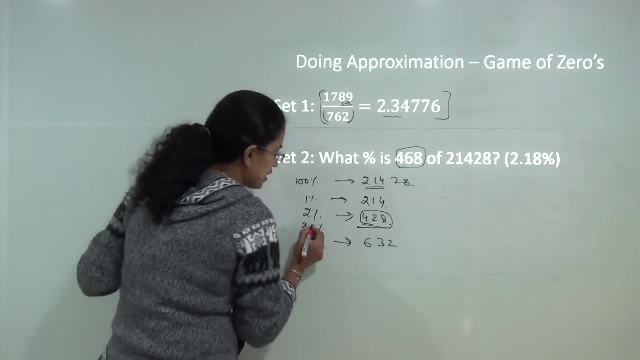 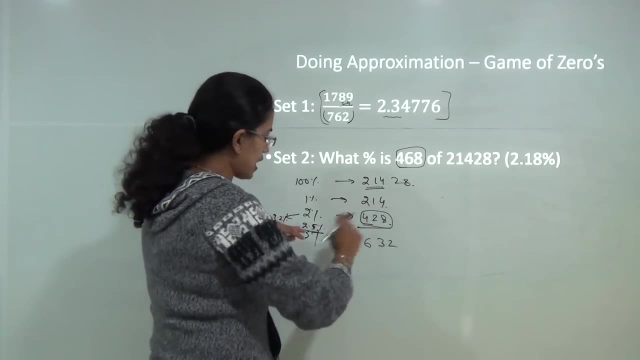 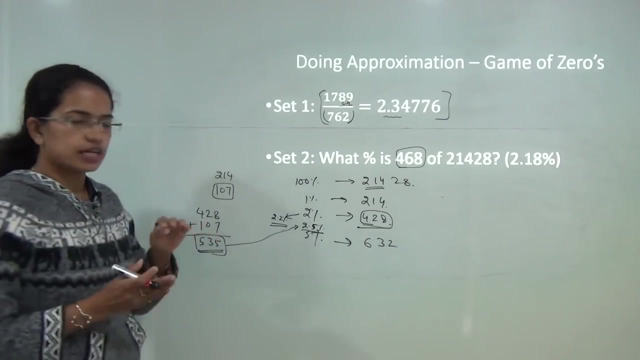 need to come on to. that means my answer would be closer to somewhere, which would be 2.2 percent, nearly, because it's far from this, and closer to 2.5 is 335, which is again a big, bigger, much bigger number than this. 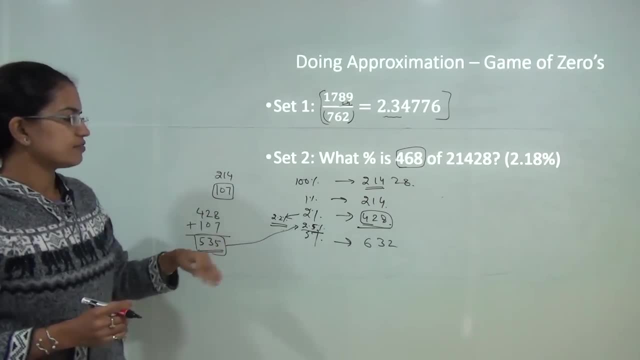 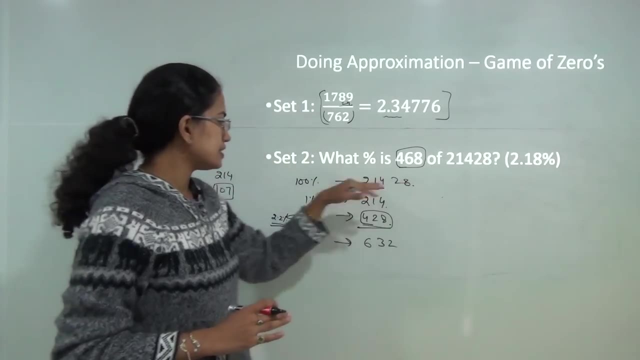 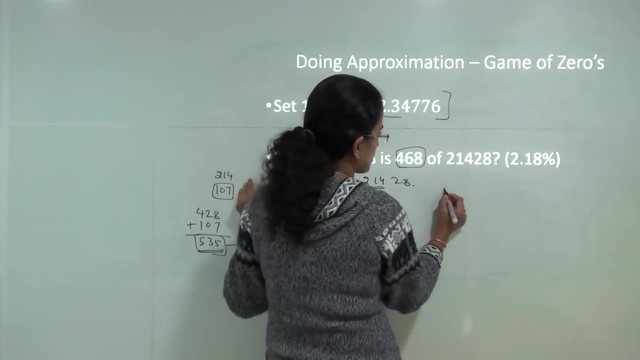 So I have 335.. So my answer would be closer to nearly 2.2 and the exact answer, as you can see, is 2.1. so that is another technique of approximation that you use here, rather than solving the complete sum. if you solve the complete sum, you can say 468 divided by 21428 into 100. 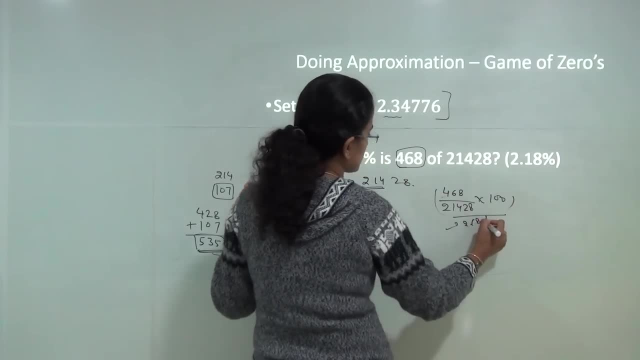 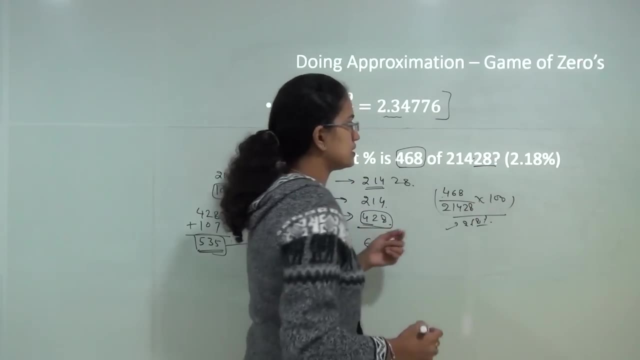 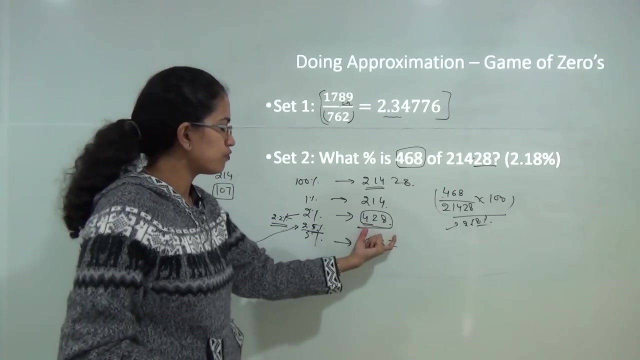 and then you solve the values and you say it would be nearly 2.18 percent. So, rather than doing that, you are trying to simplify it. it because, if you put the decimal place here, ignore the last digits, since they are smaller than 0.5. you take 214, double 214, that is 428, and you are going. you need to go close to. 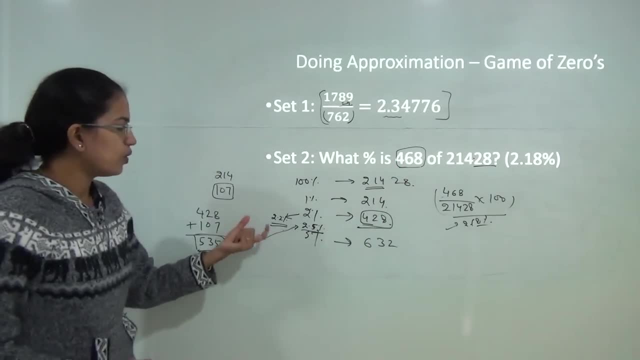 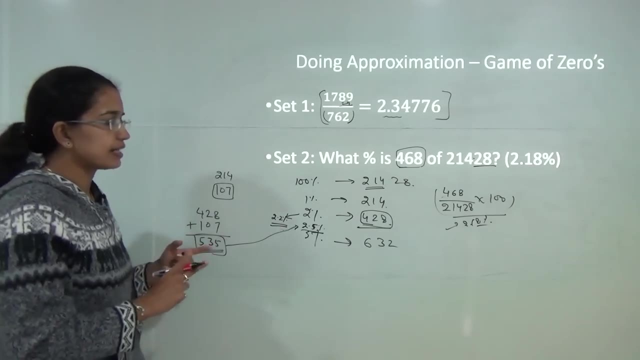 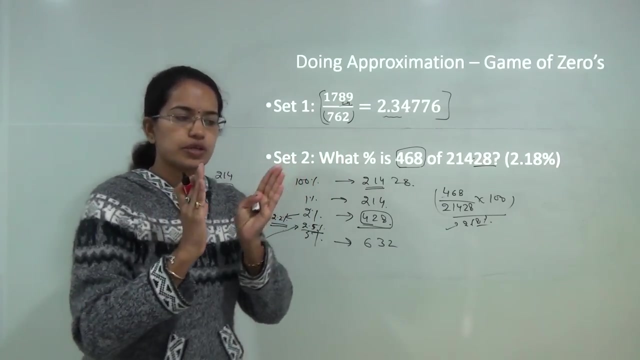 468, so that means you will go somewhere around 2.2%. as you can see here we have calculated 3% and 2.5% for better understanding. and these type of question when you solve once or twice you will have a kind of good visualization to get closer to approximations much quicker. 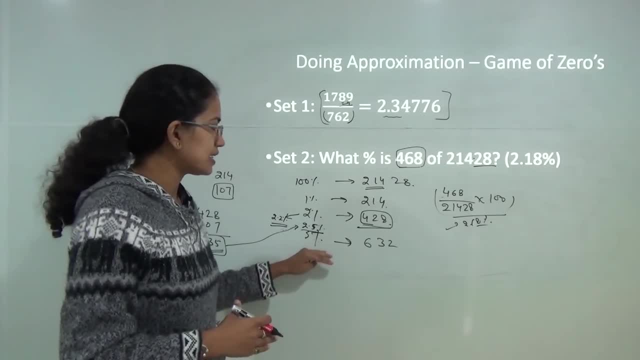 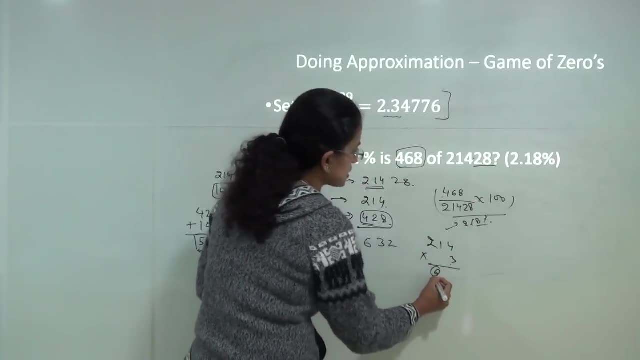 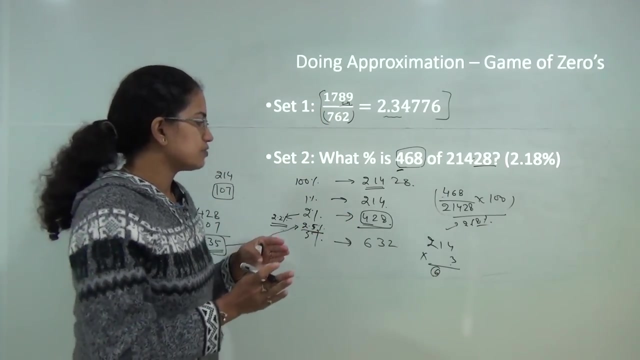 so in the first round you might calculate 3%, but in the second round you would have an intuition that if I do 214 into 3, this digit would be 6 and this, if this is 6. this is very far from this, so that my answer can never be towards 3, so my answer would be closer. 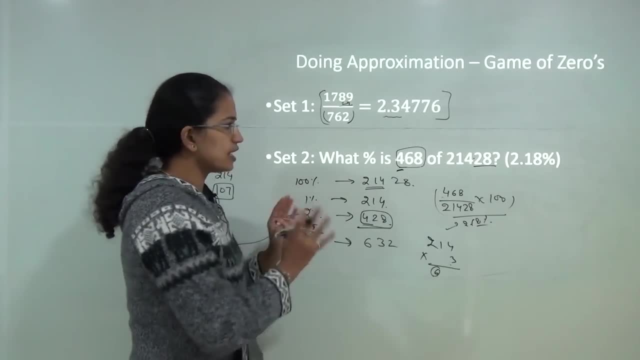 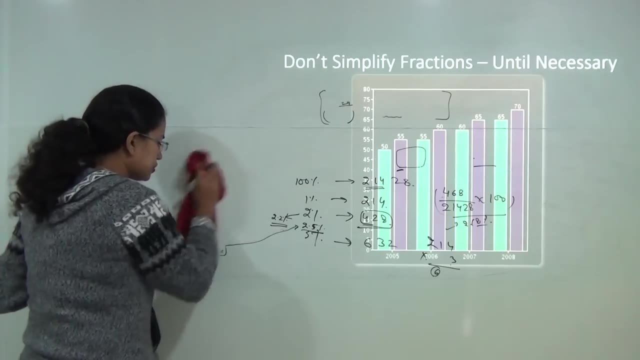 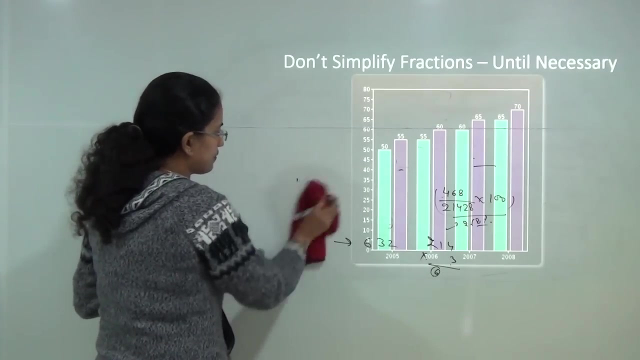 to 2 in all possible cases. So these are the way you need to do approximation. Now, when it comes to fraction, I usually recommend: do not solve the fractions, keep the fractions as it is until necessary. so, if it is necessary, if the answer is given only in decimals, then 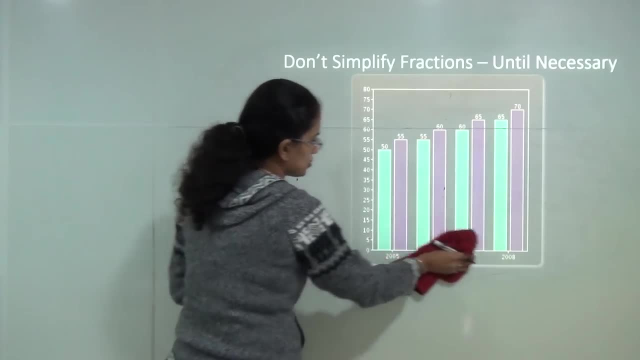 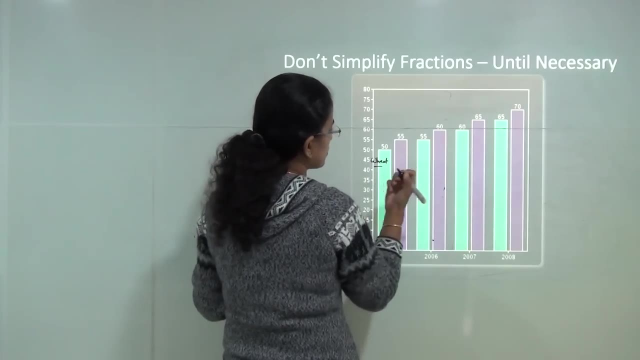 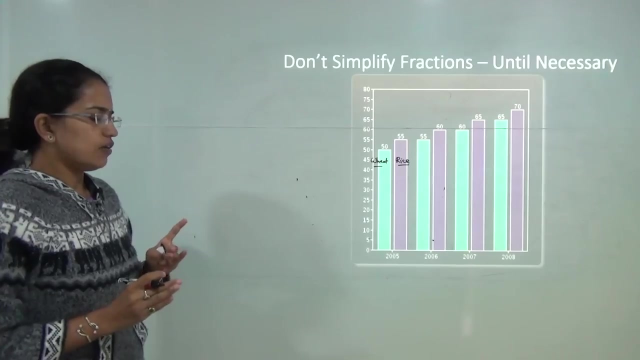 definitely go ahead and solve the fractions, otherwise there is no need to solve the fractions. Now let us say: the blue bar denotes the wheat production and the pink bar denotes the rice production. Now, in which year Was the wheat production highest? now, whenever a question like this is asked, what is what? 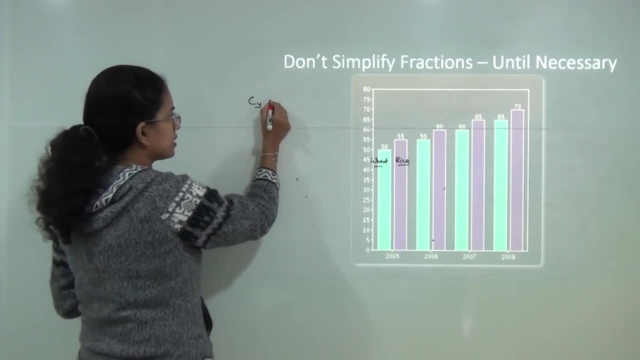 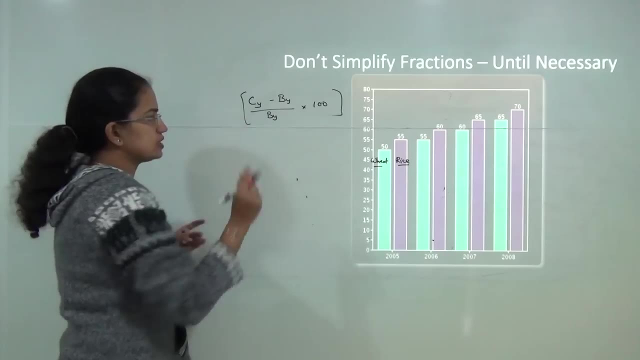 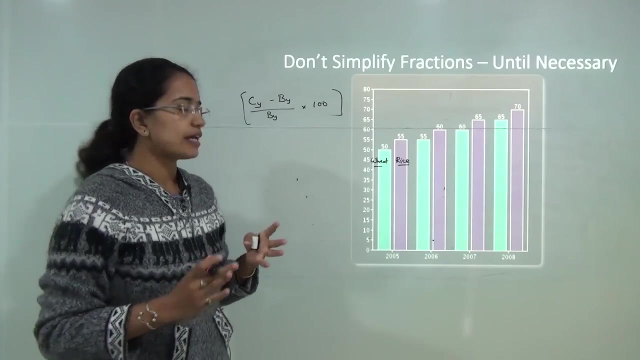 you have to do is you have to do the current year minus the base year, divided by the base year into 100, and this is another standard formula that you must remember for all data interpretation questions you might have come along with binomial problems and binomial 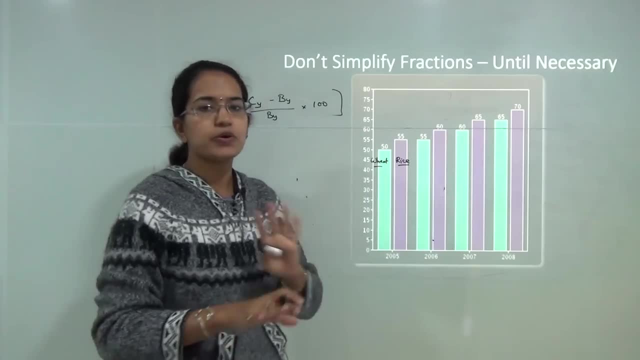 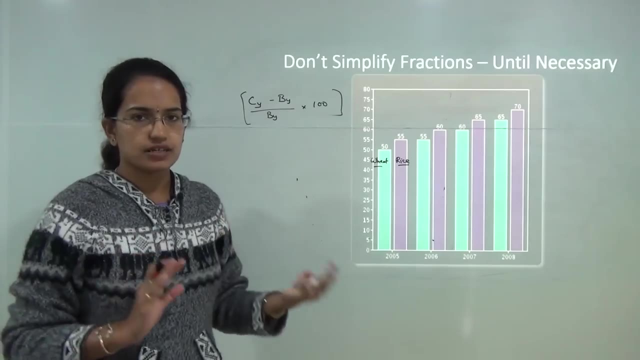 equations which help you solve the growth rate problems, but do not go into that detail. You can simply solve the questions with a simple formula. that is current year minus base year, divided by base year into 100. now, if you remember this formula and you try to, 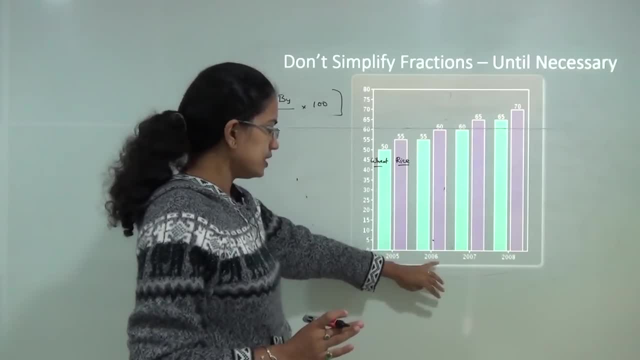 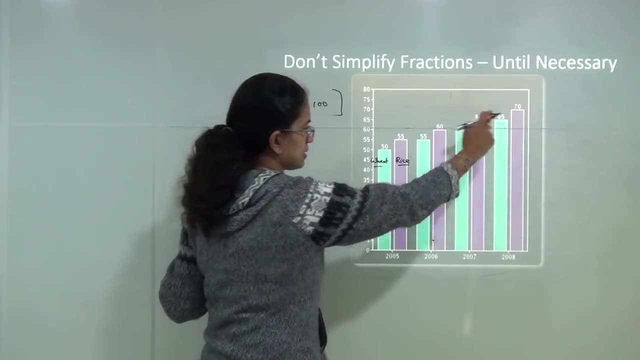 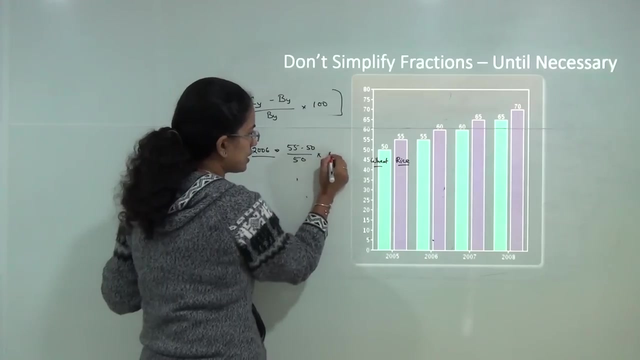 apply it universally. now what would happen here? let us calculate it for 2006. what would happen? wheat production is 50, 55, 60 and 65. so let us say for 2006 it would be 55: 50 divided by 50 x 100. 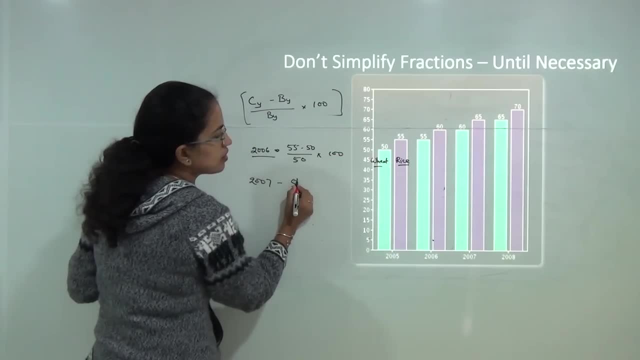 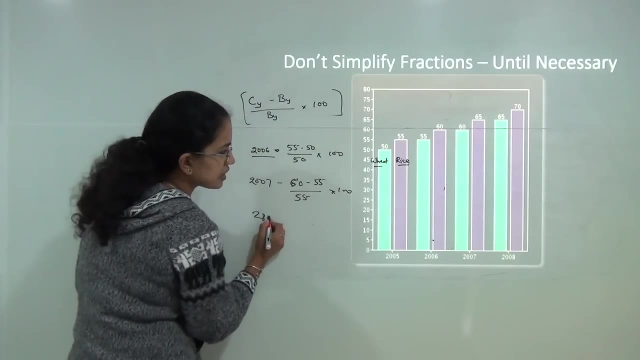 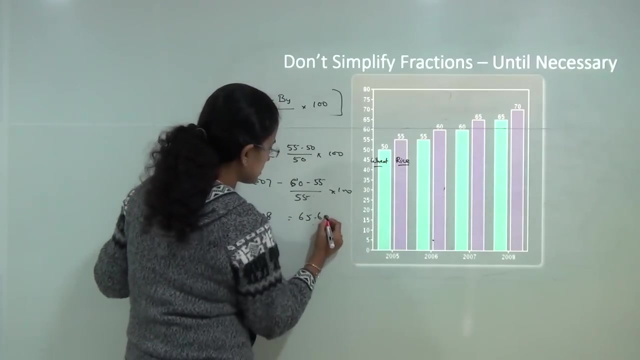 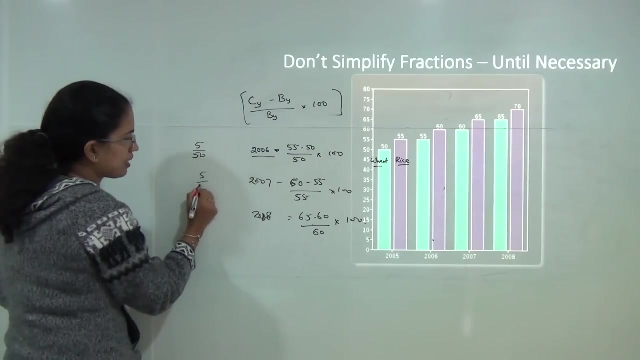 2007 it would become 60-55 divided by 55 into 100, and for 2008 it would become 65-60 divided by 60 into 100. now, if i simplify this, it would be 5 by 50, it would be 5 by 55 and it would 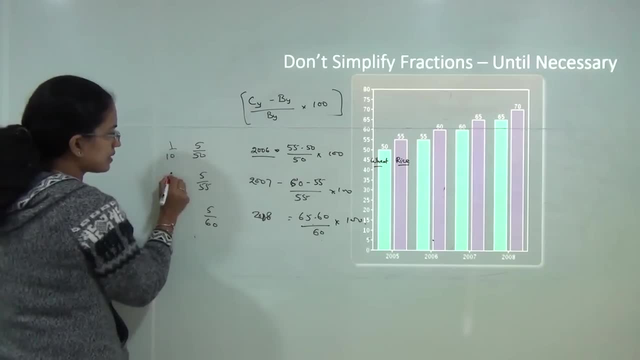 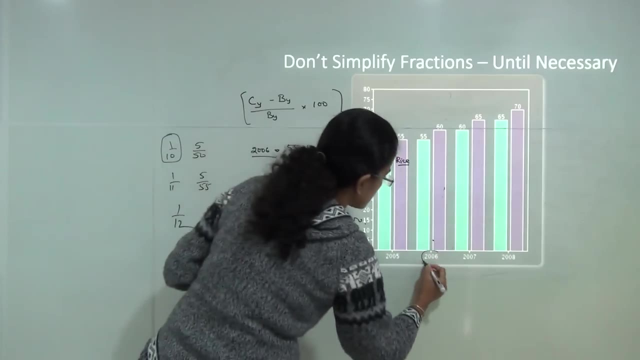 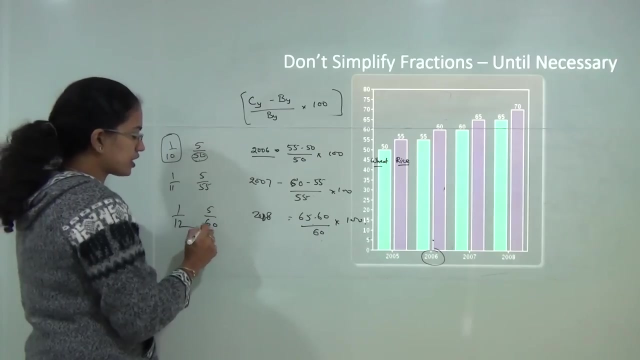 be 5 by 60, again simplifying 1 by 10, 1 by 11 and 1 by 12. so i can say the highest production would be in year 2006. why? because if you have higher numerators- sorry, higher denominators- 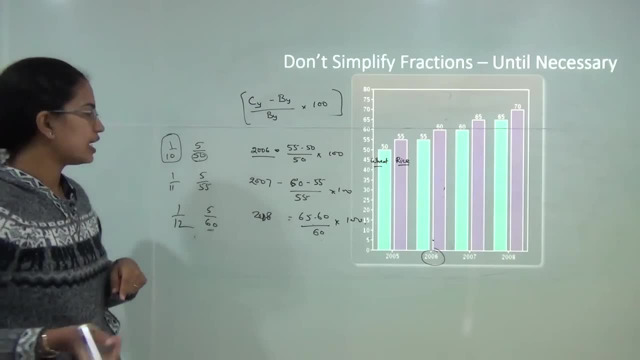 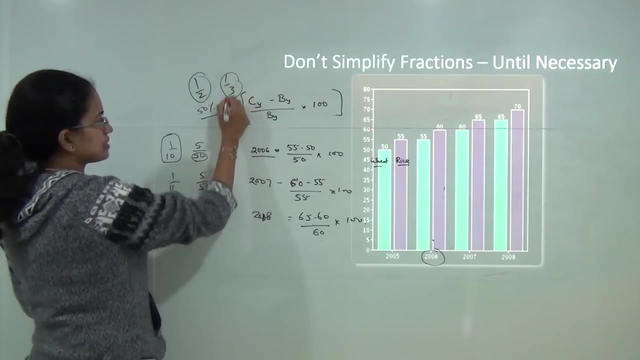 the fraction would decrease and it would be lower in the answer. because if i simply say 1 by 2 or 1 by 3, i can say 1 by 2 is nearly 50 percent and 1 by 3 is nearly 33 percent. 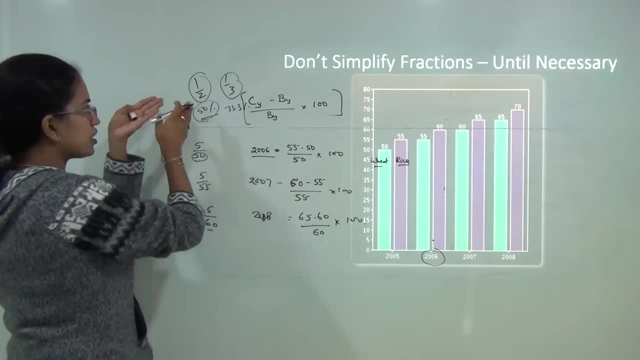 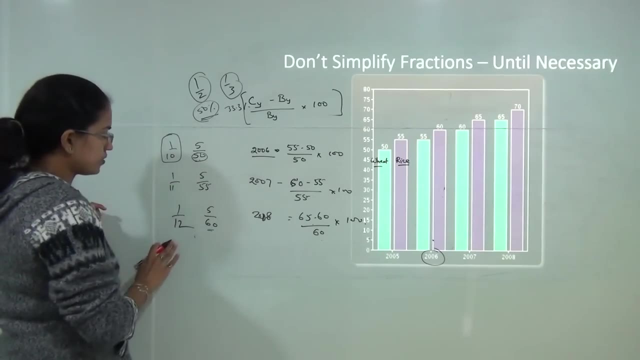 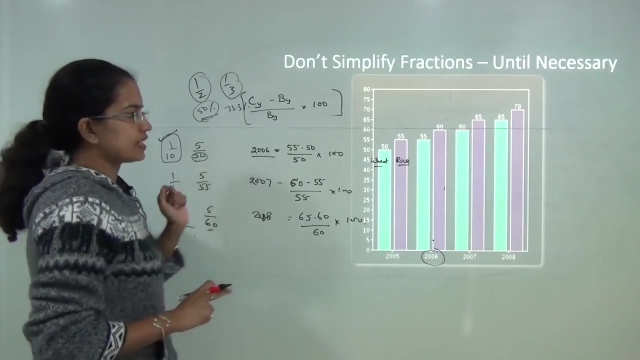 that means 1 by 2 is bigger. so if your denominator is smaller, your answer is bigger. so if your denominator is smaller, you will have a bigger answer and therefore highest value of production would be in the year 2006. similarly, if it asks about rise production and which year, 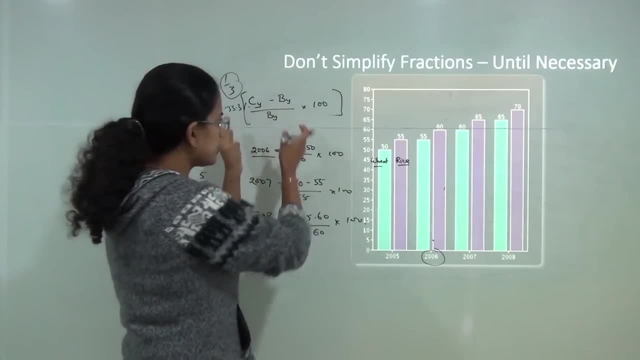 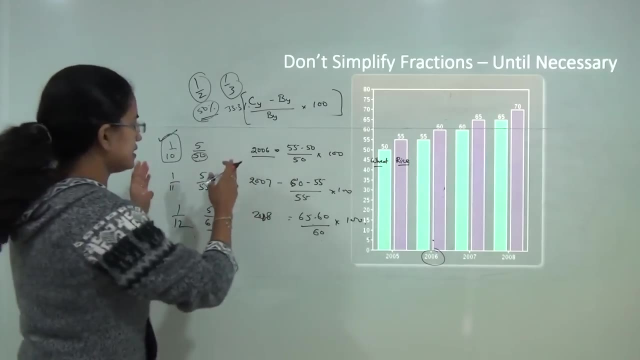 would have the lowest rise production. you will again do the same thing, current year minus base year by base year into 100. you will do it for all and you will have the same answer. and let's say you come up with the similar answers so you would have for the 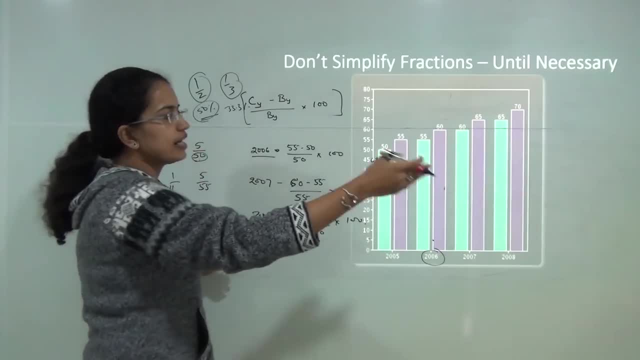 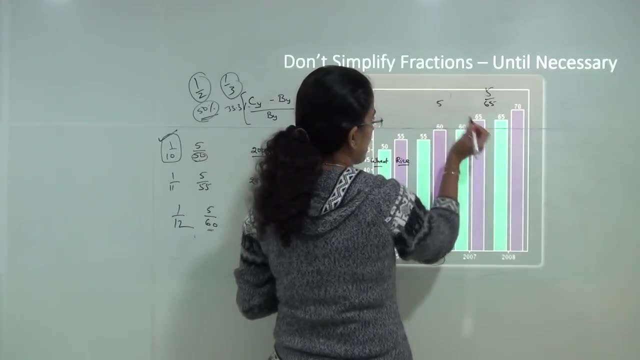 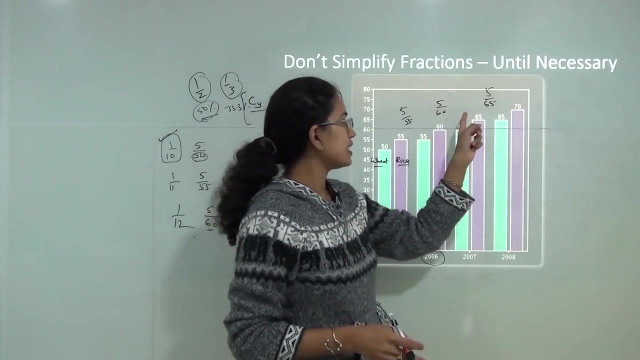 last one, you would have 5 by 65 into 100, and that 5 by 65 would be the lowest fraction, because in this case you would have 5 by 65. in this case you would have 5 by 60. in this case you would have 5 by 55. so these would be the three ones for the rise, and then you 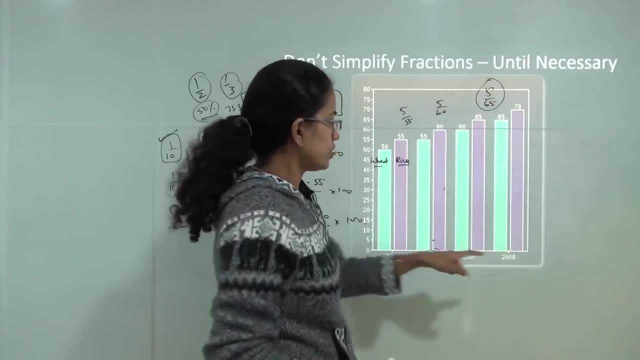 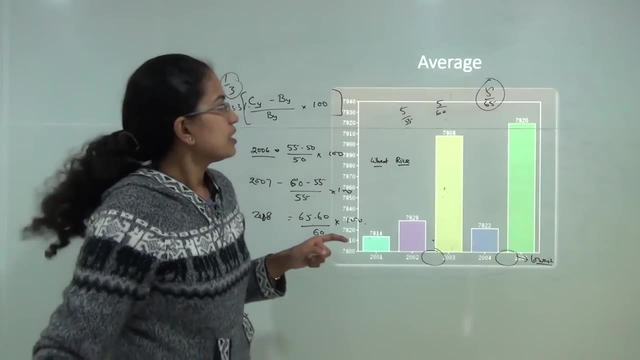 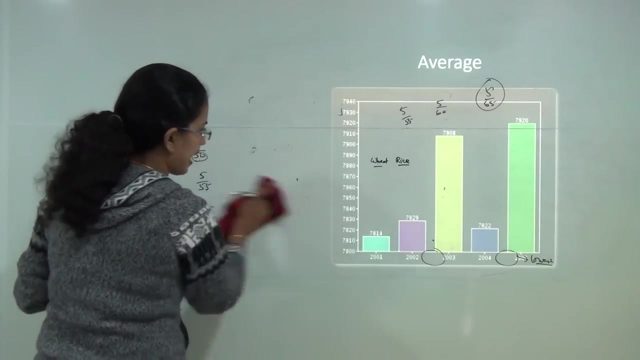 can say this would be the lowest among the three, so year 2008 would have lowest increase in the rise production That could be visualized now. next question is: sometimes there is question that is asked to calculate averages. now, when you need to calculate the average, there is an interesting 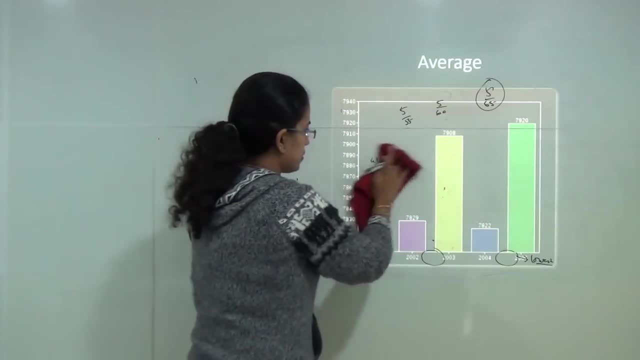 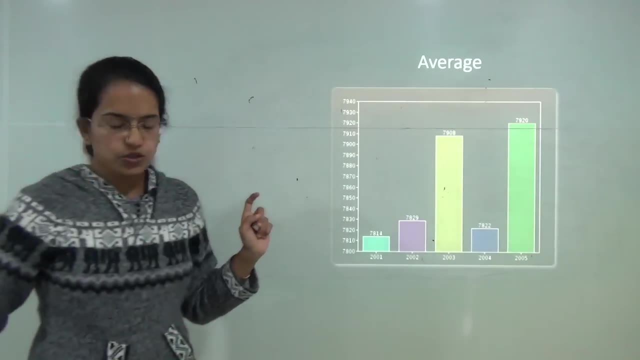 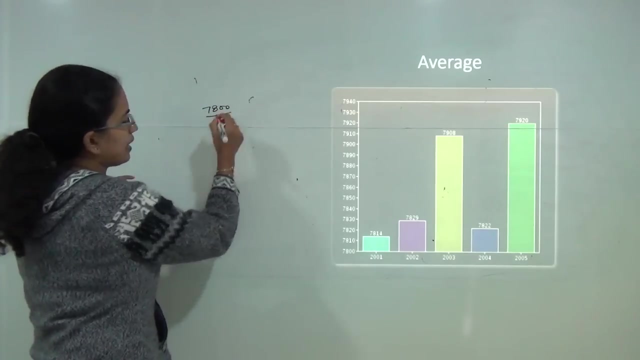 thing that you must understand is you must look into the figures and see if they are close to one another. so, for example, let's say this graph: you have all the figures that start with 7800. now if I take away 7800 and work around this figure, you will see that this is. 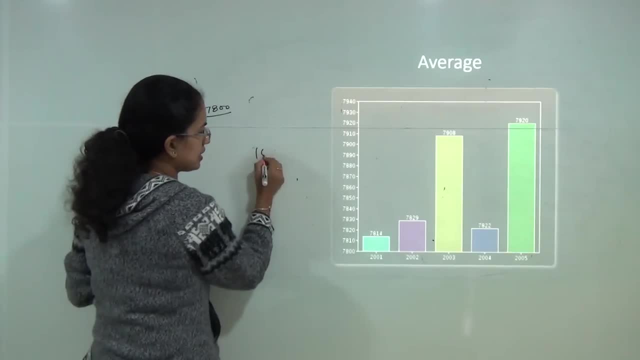 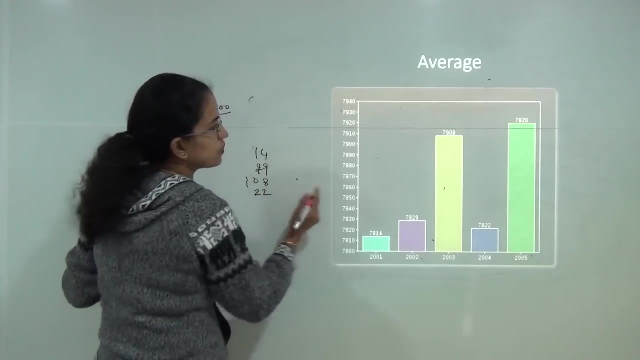 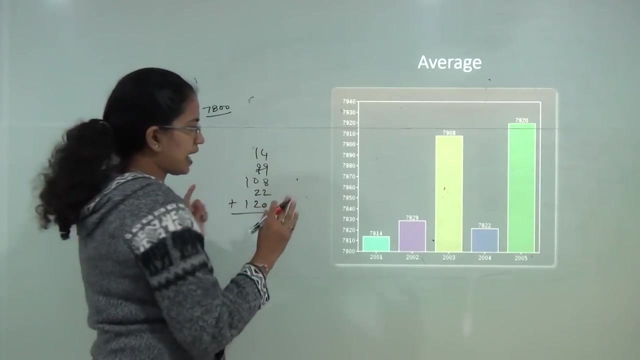 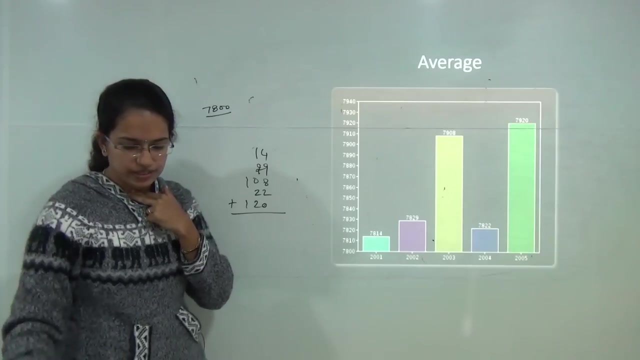 the average. So this is the average of all the remaining ones. so you have 14 here, you have 29, then you have 108, then you would have addition of 22 and finally addition of 120. that means you will add all the remaining values except 7800. so when you add all these values, you 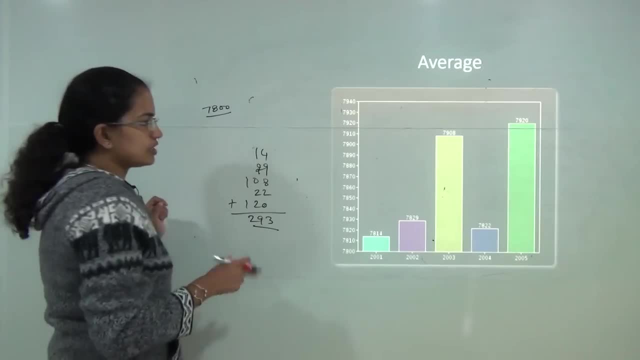 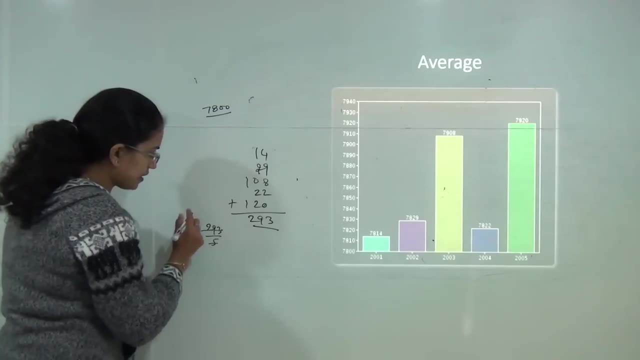 get an answer of 293.. Now this 293 is the average of all the figures. So this is the average of all the figures. So this is the average of all the figures. So this is the average of all the figures. So 293 is divided among 5. so 293 divided by 5, I can simply say 5 x 5 is a 25 and 4 carry. 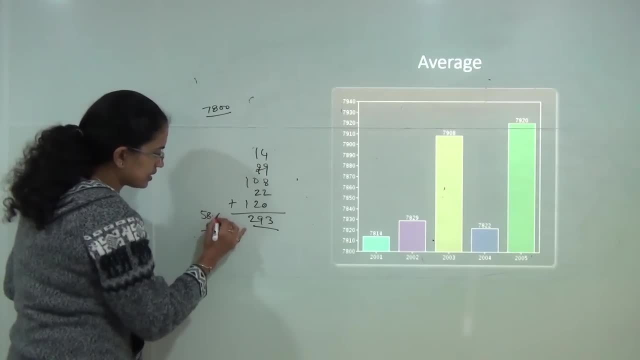 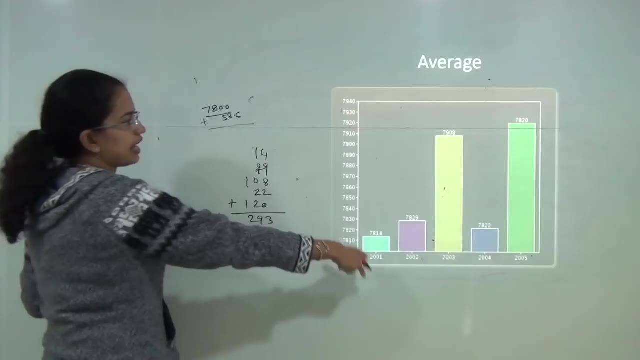 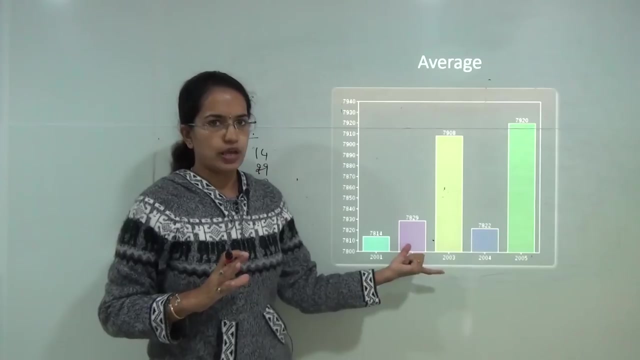 over. so you would have 8.30. that is 6, 58.6. now this 58.6 I can add on to this. therefore, the average of all these values would be 7858.6.. So that's a simpler way to calculate the averages rather than going into the details of each. 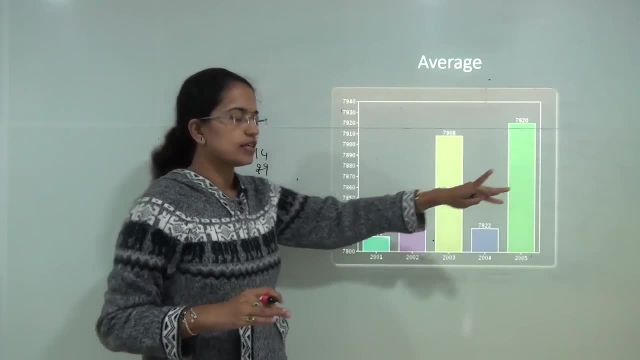 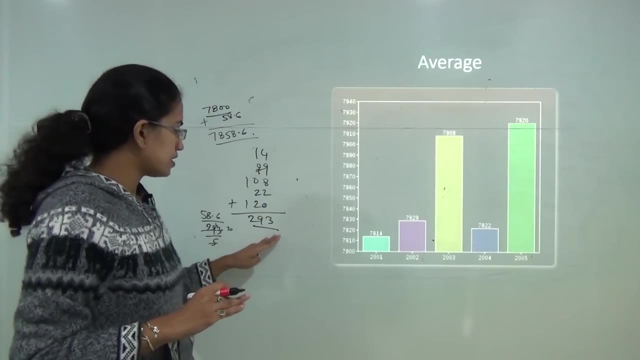 of each and every one thing, adding all the values together. what you can take aside is take the common values out and then add the remaining values. when you total out the remaining values, take a average of the remaining values and add that value to the base value that. 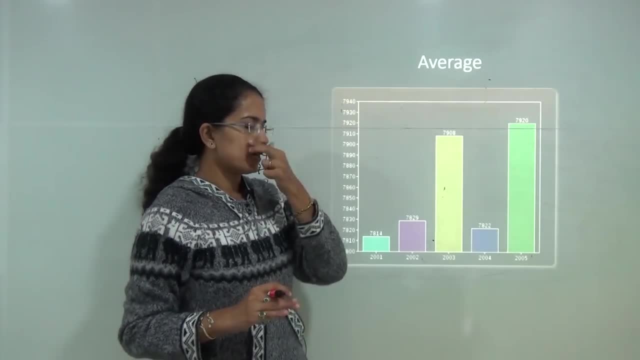 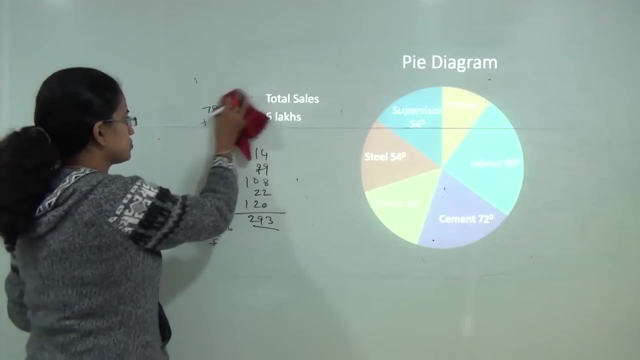 you had separated in the starting. So that is how you work around quickly with the averages. Now. the next thing is pi diagram. now this is a main area where most of the students are struck up. the simplest thing I would say here is: you have to remember two things. 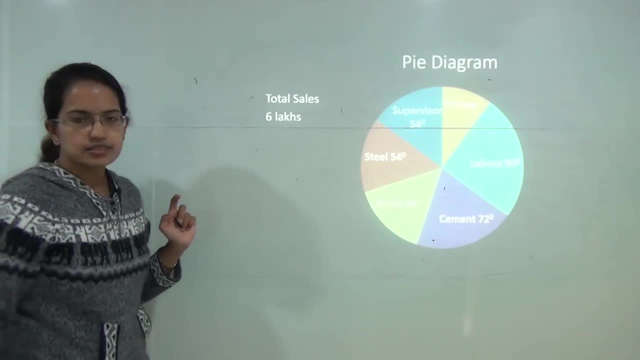 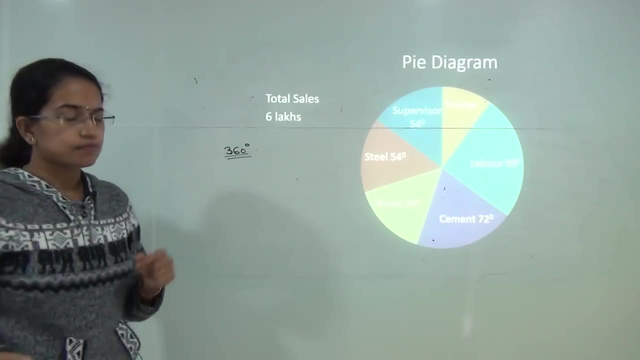 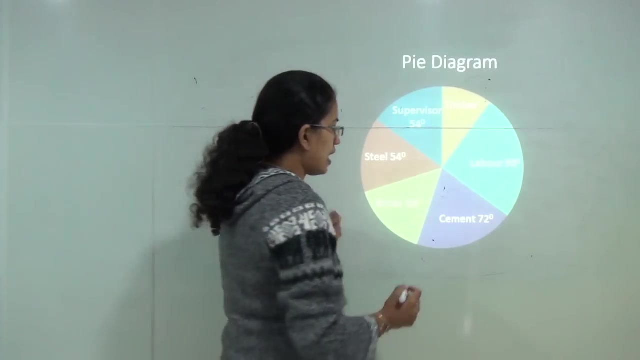 first of all, a circle makes 360 degrees. that is the basic key. and once you know that circle makes 360 degree, you can solve each and every problem. Now, what is given here is: the total sales is 6 lakhs and if it is asked, what would be? 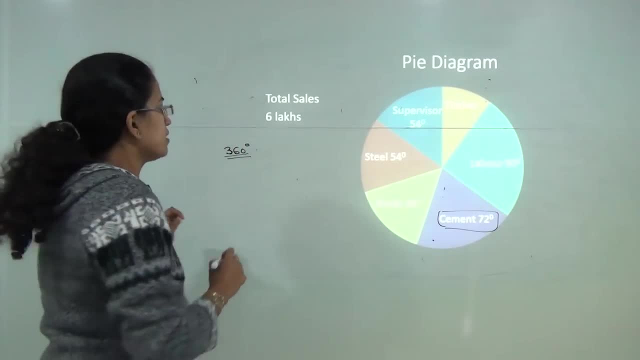 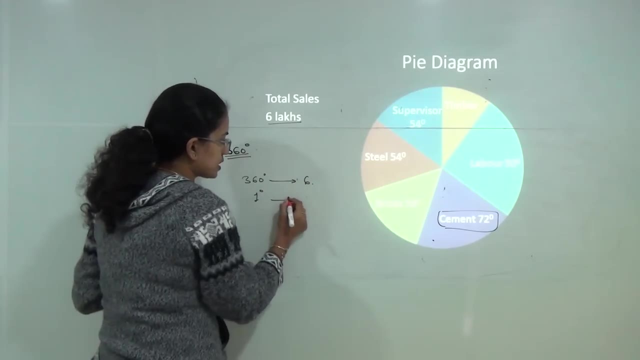 the sale of cement. how would you calculate this? when I say total sale is 6 lakhs, I can say: 360 degrees give you sale of 6 lakhs. So 1 degree would give you sale of 360. sorry, 6 by 360, so 72 degrees would give you a sale. 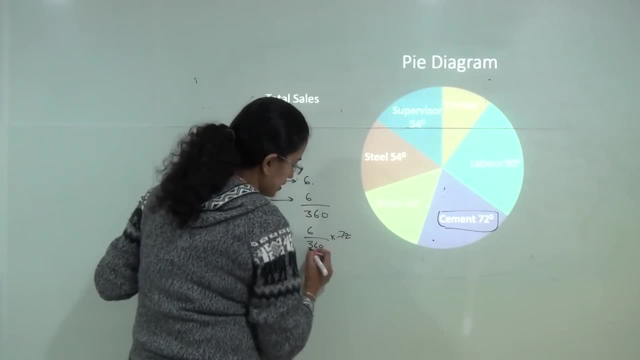 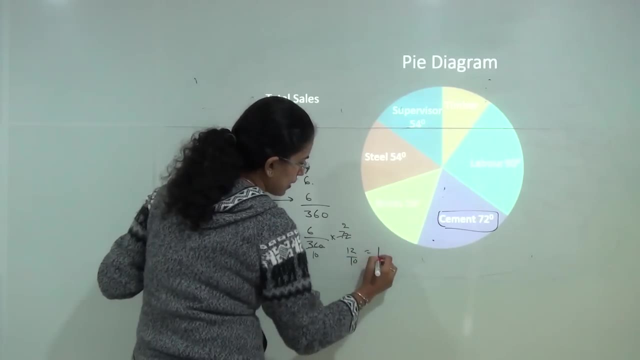 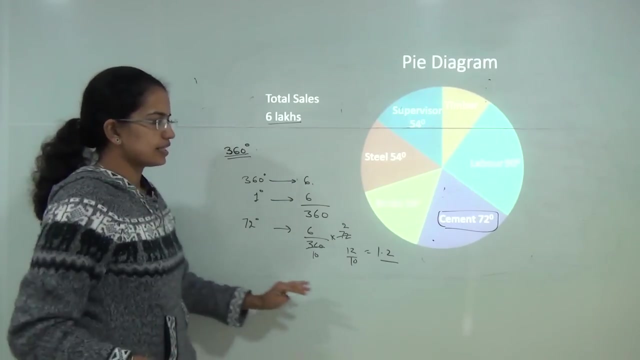 of 6 by 360 into 72, 36, 10, 2, and then you would have 12 by 10, that is 1.2. so I can say the sale of cement would be 1.2 lakhs. now this is again a simple, unitary method that you 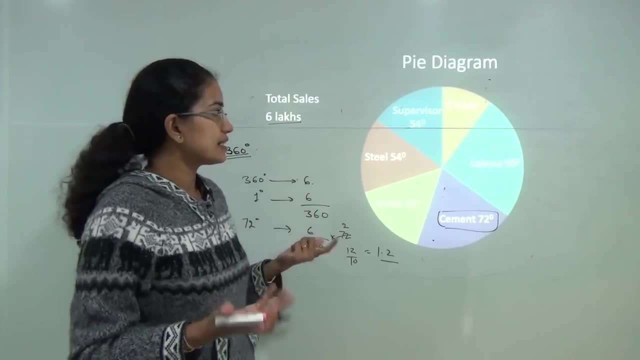 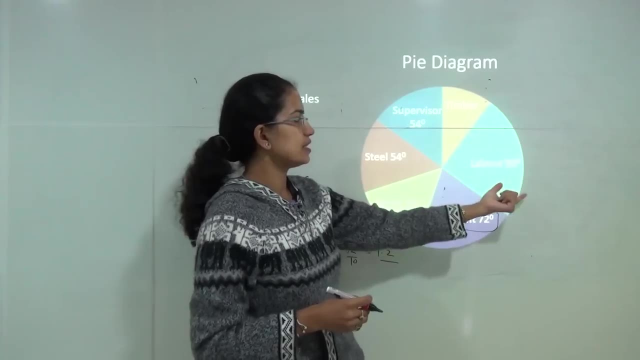 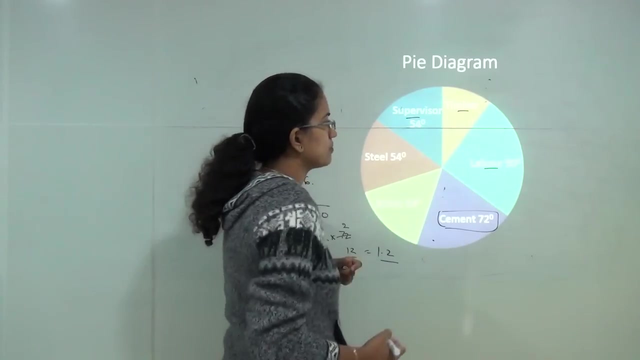 need to apply When you are given with degrees. now, another interesting question would be: what would be the percentage of sale if I take supervisors, timbers and labours together? now, if I have supervisors, timbers and labour together, I do not know what is the degree for timber. 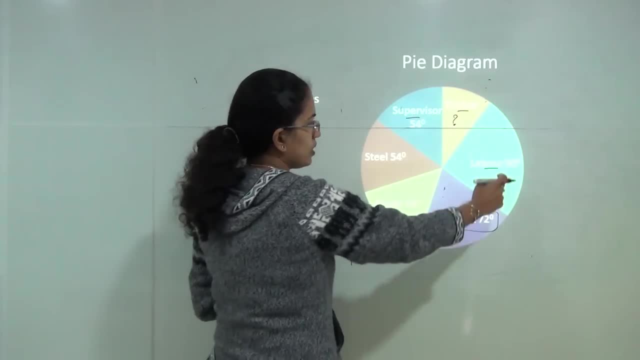 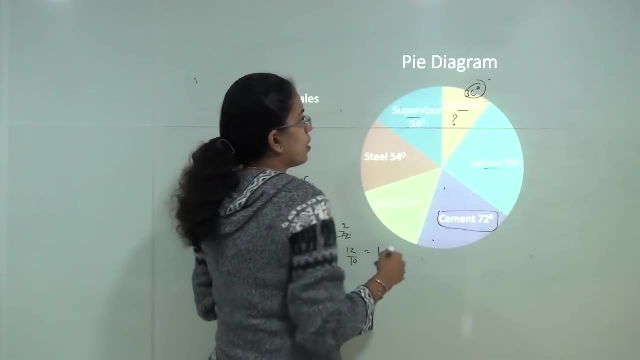 so first of all I need to calculate that. so I will add up all the remaining degrees and subtract that from 360, so that will give me the answer, for timbers is 36 degree. Now it is given that the sale of these three together would account for what percentage. 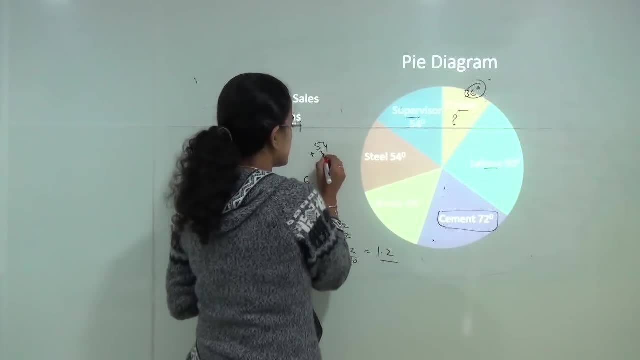 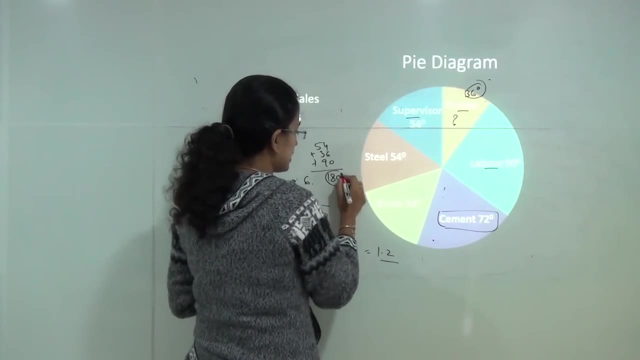 of the total. that means 54 plus 36 plus 90. so it gives you 54 plus 36 is 90, 90 plus 90 is 180. now this 180 out of 360 accounts for what percentage? so I can say it would simply: 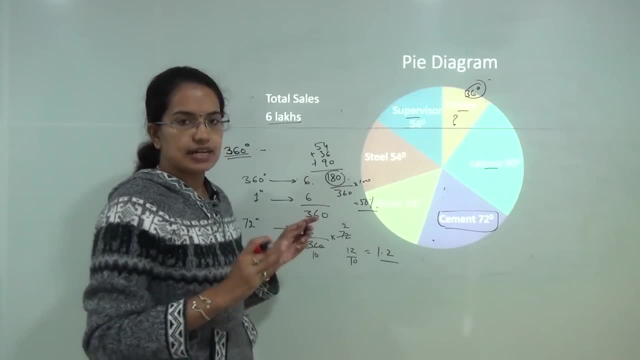 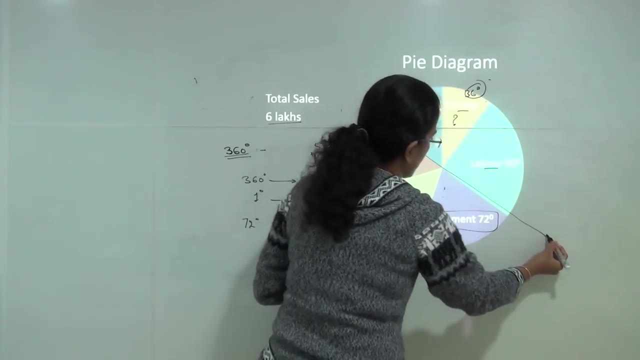 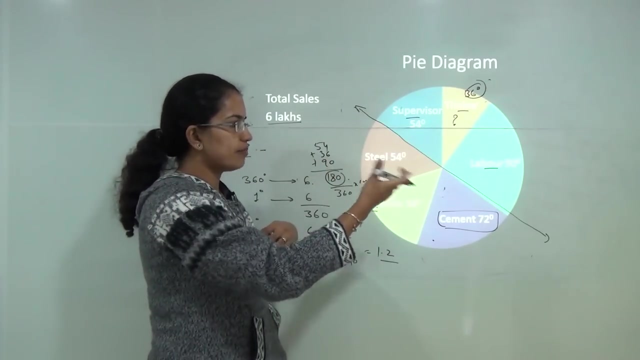 account for 50 percent of the total and if that graph is drawn to the scale, you can simply calculate that. You can simply say: here this line denotes 50%, so 50, 50- this line denotes the breaks the graph into the pie chart, into half. so you have 50% on that side and these three 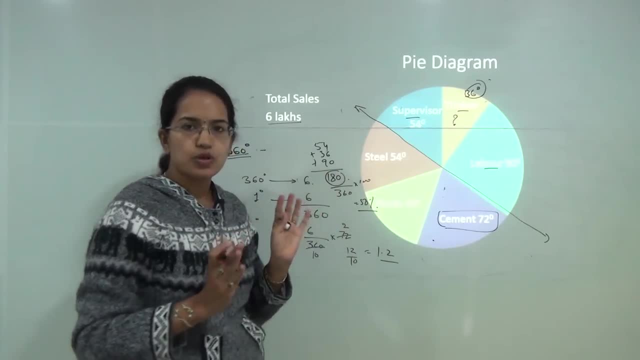 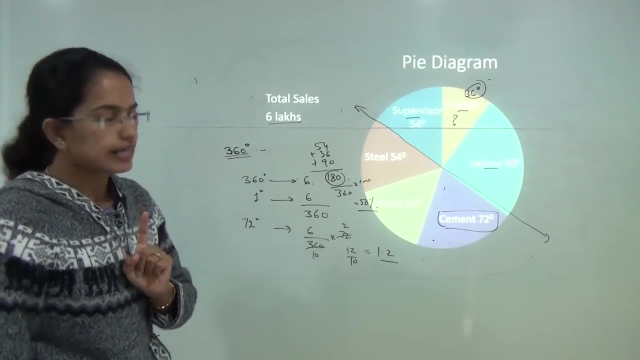 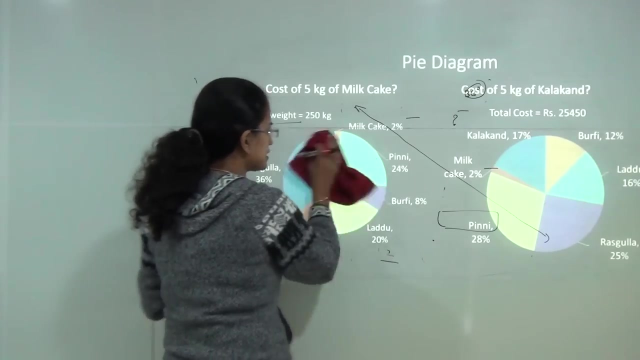 would again make up 50%. so that is how you solve problems like these for pie graph. so this is the first example for pie diagram where you are given degrees. the next case we will take is a bit complicated and you must understand this carefully. Now, to solve problems like this, there are n number of methods given n number of books. 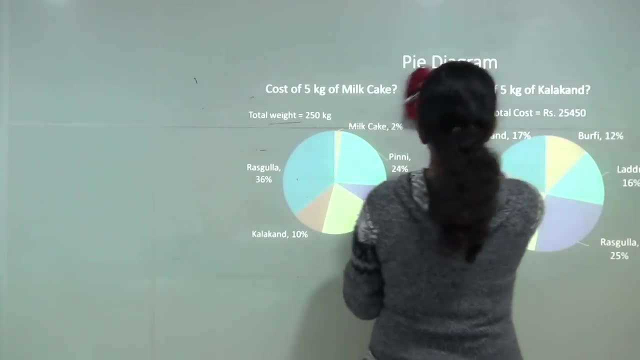 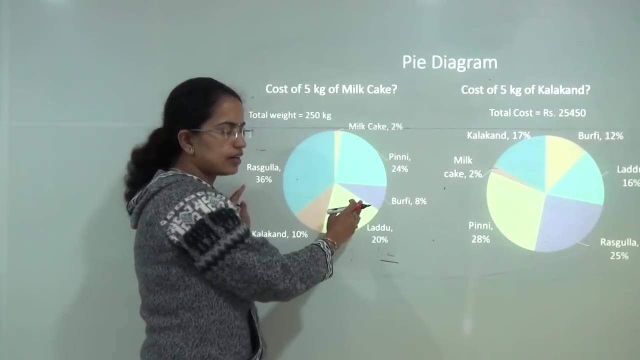 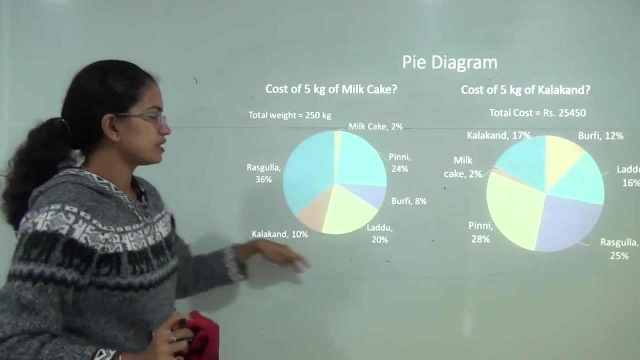 that you can refer, but what we will work around is a simplest of all. what is given here is you are given the total weight of the sweets that is available at sweet shops. that is, the total weight is 250 kg and you have given the proportion of the weights for each of. 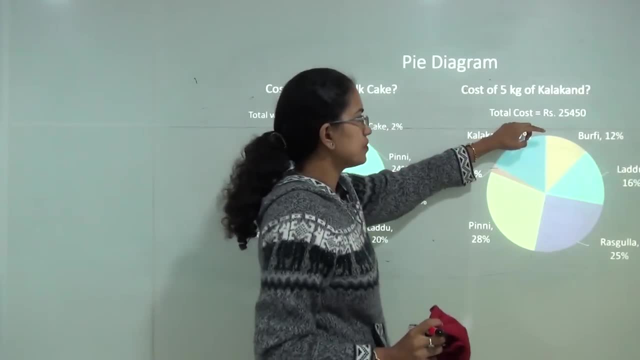 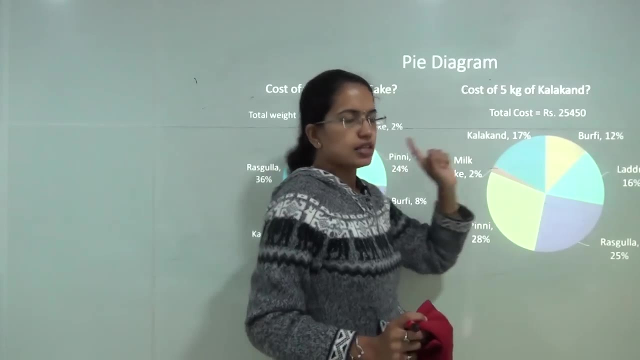 these. you are given the total cost of the sweets, which is 250 kgs. You are given the total cost of the sweets, which is 25450, and you are given the individual percentage of the cost. Now, if you are given to calculate the cost of 5 kg of milk cake, how can you do that? 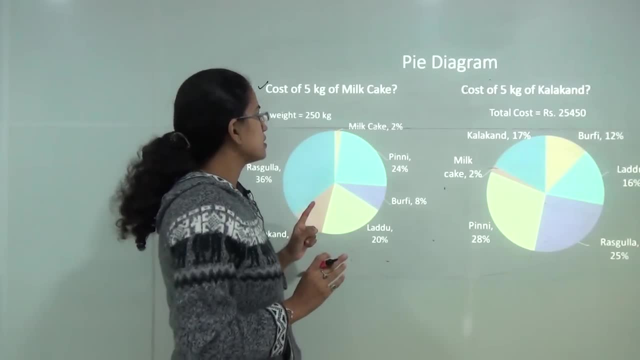 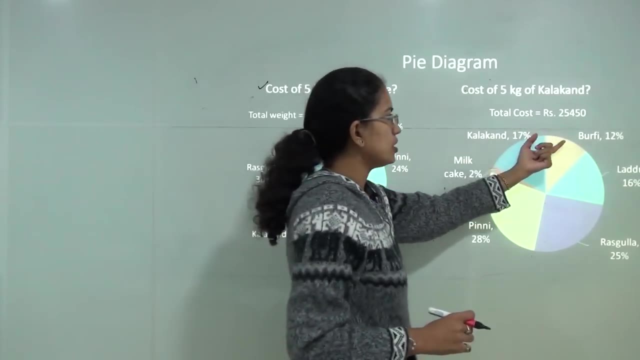 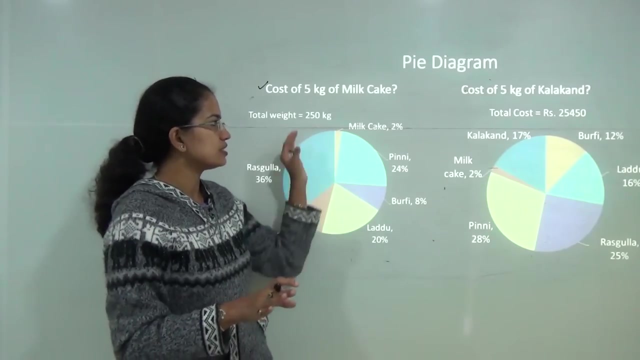 Now, the first and the foremost thing that you need to understand here is you have to see if the ratio or the proportion of weight and the proportion of cost is same, then you know. you don't need to go further into the details, you can simply solve it with one. 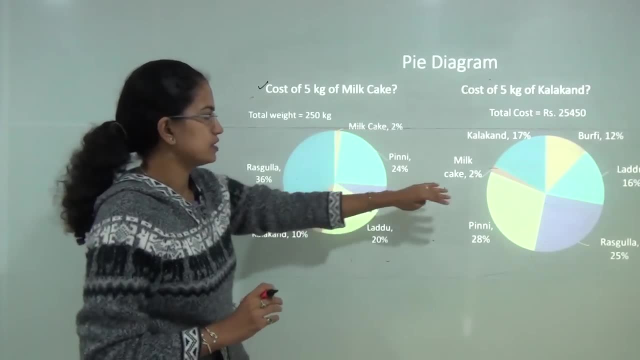 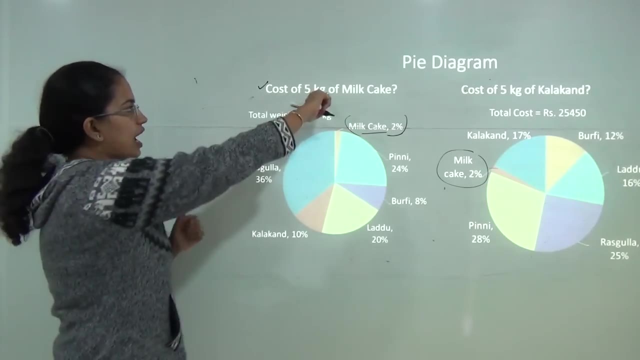 step. Let's say we will do it for the milk cake first, because it's 2% in both the cases. so this makes the question simpler. Now we will work around for milk cake and you are asked to find out the cost of 5 kg. 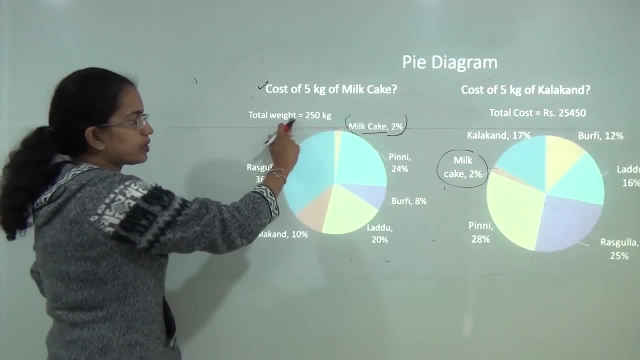 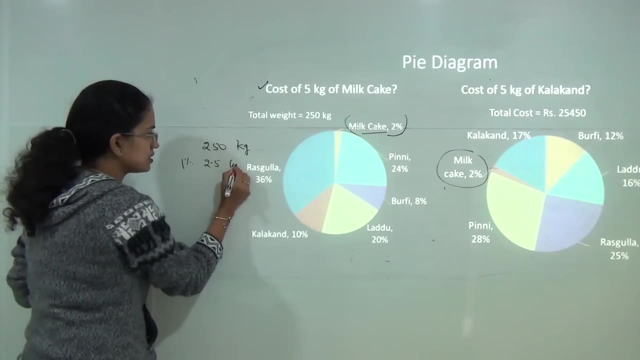 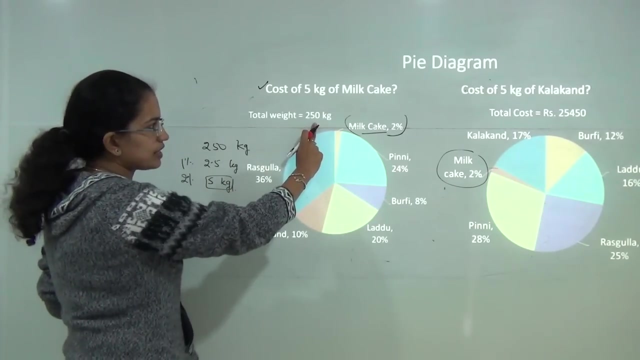 of milk cake how you can do that. The total weight is 250 kg. Now 1% would make 2.5 kg And 2% would make 5 kg. Now, if I know, the total weight is 250 and the total cost is 25, so 250 kgs. bear you a. 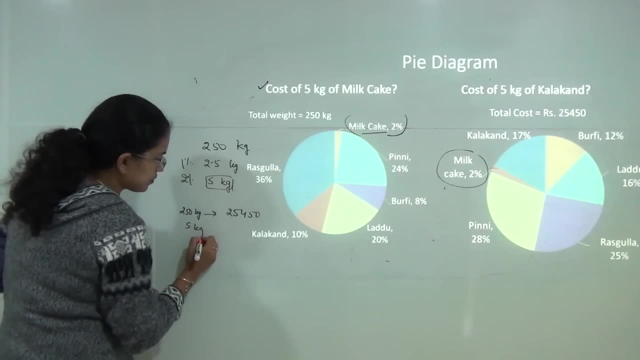 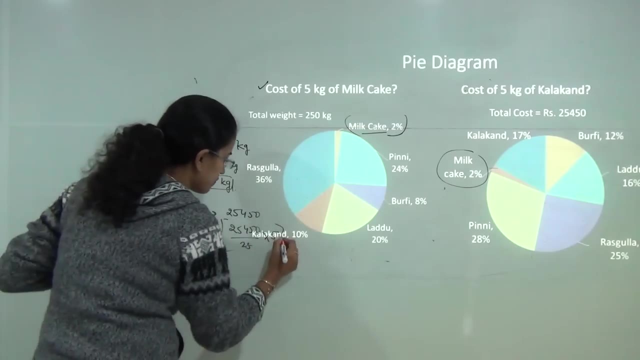 cost of 25450. So 5 kgs would bear you a cost of 25450 divided by 25 into 5. so that's one way of solving it. Another way of solving it is: Since you have 5 kg of milk cake. 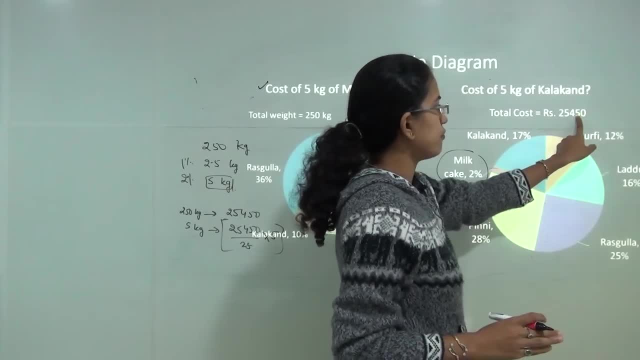 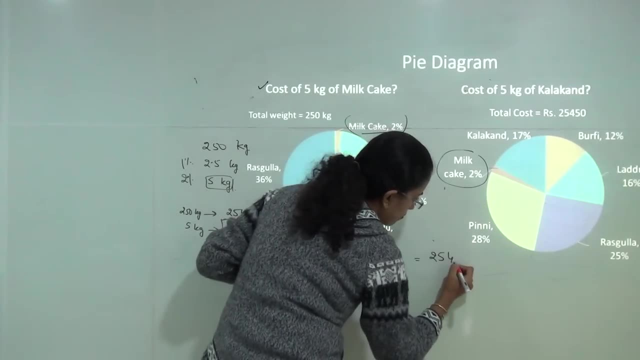 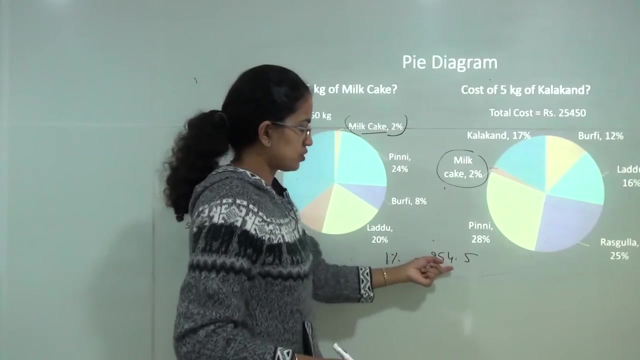 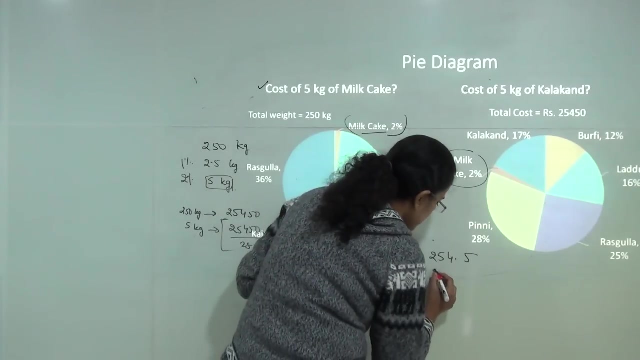 Since the total cost is 254.5, for 1% it would be 254.5. so for 2% milk cake it would be double of this. so 250 and 250 is 500. 4.5 plus 4.5 is 9. so 500 plus 9 is 509- again a shortcut. 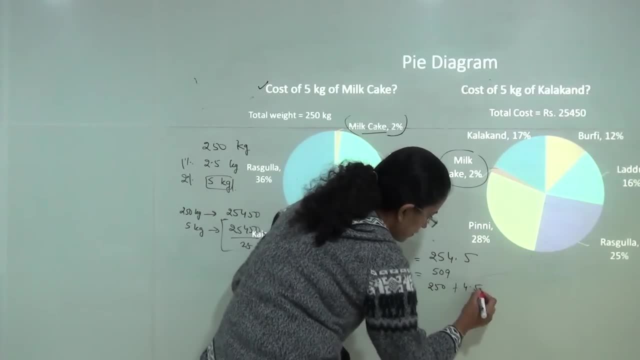 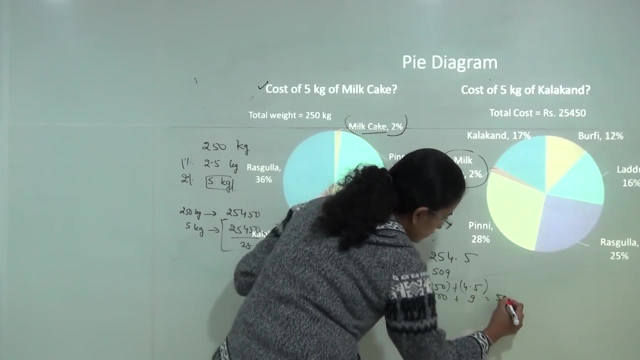 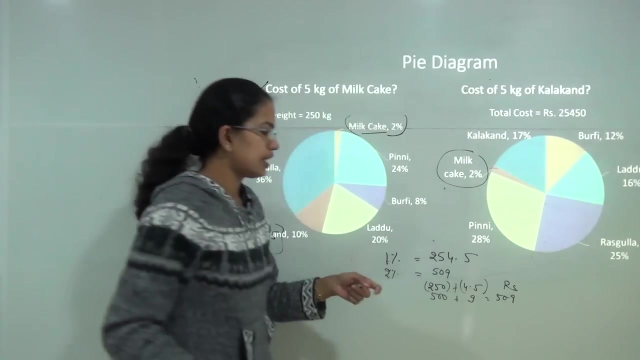 to solve this. So I broke this into 250 plus 4.5. I double this and I double this individually, so this becomes 500 and this becomes 9. now I add this, so it is 509.. Now so 2% would have a direct cost of rupees 509, and if I calculate this, I would again. 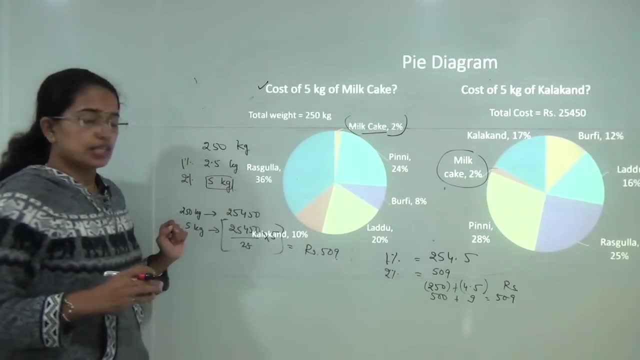 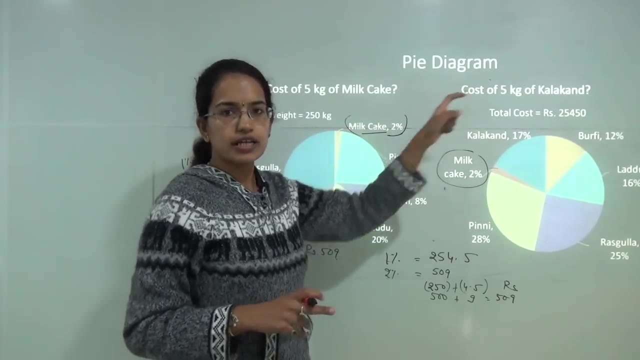 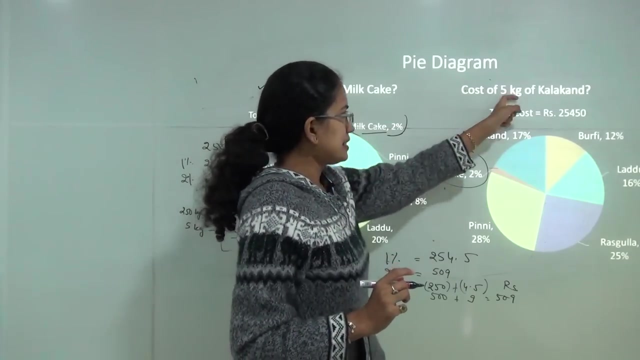 get rupees 509 as the answer. So this was a very simple method to solve the problem when you have equal proportions in the cost. Now let's complicate this question further In the next set. what is asked is cost of 5 kg of kalakan. 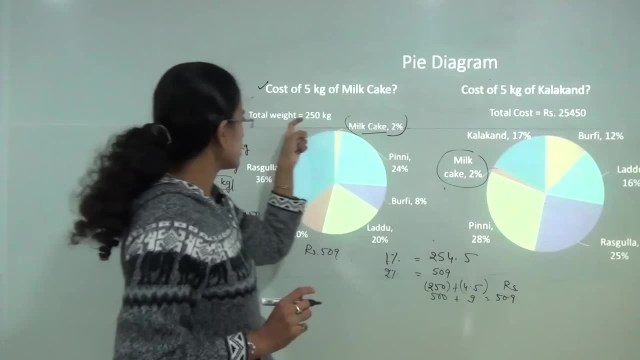 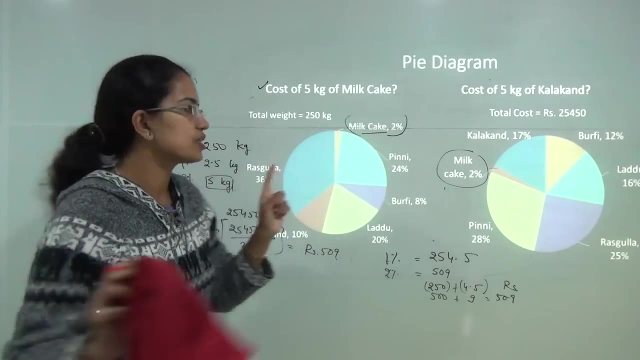 Now, when you are asked about kalakan, let's look into the weight. By weight, kalakan is 10% and by cost it is 17%. So solution for this won't be as simpler as we did it for milk cake. Now let's move on to solving this section. . . . . . . . . . . . . . . . . . . . . . . . . . . . . . . . . . . . . . . . . . . . . . . . . . . . . 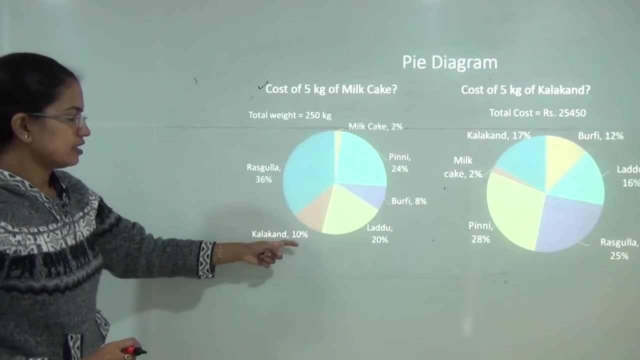 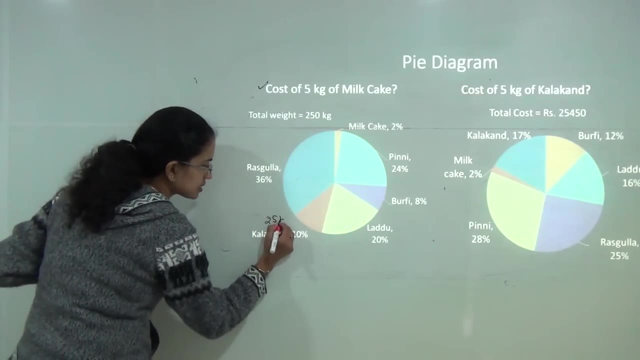 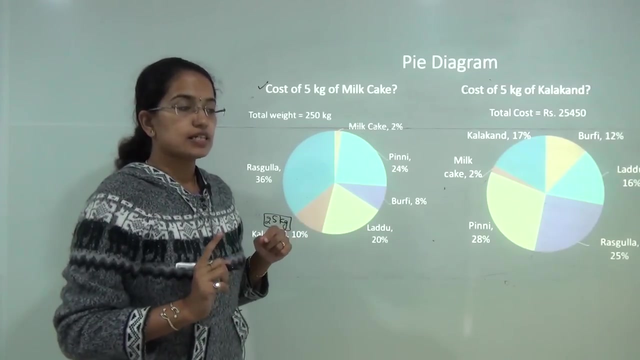 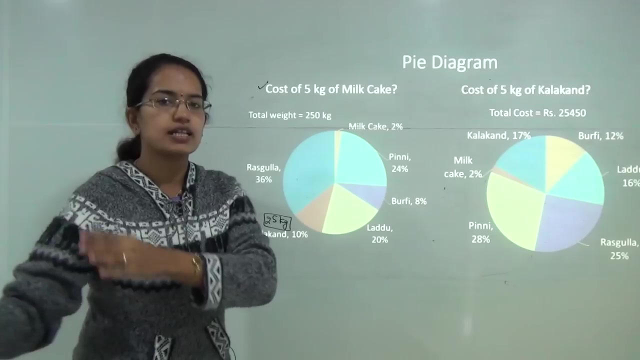 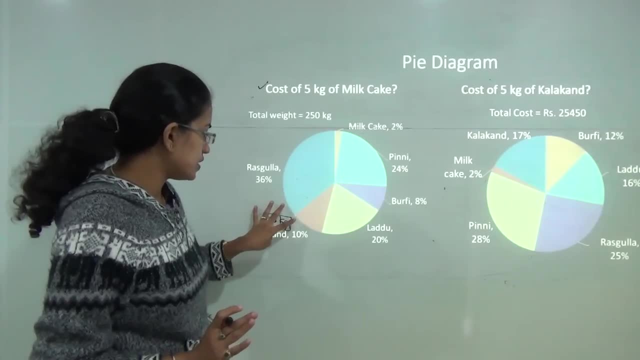 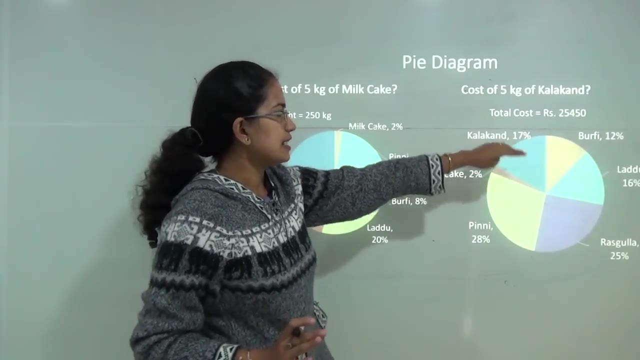 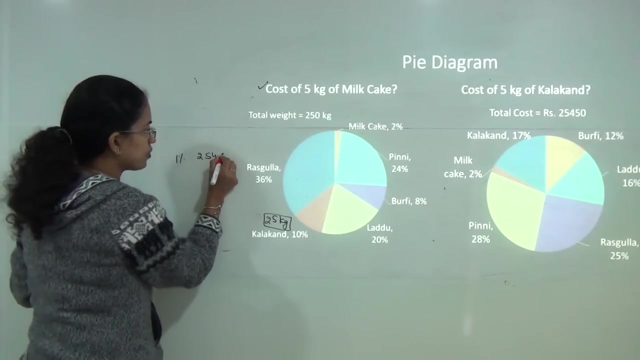 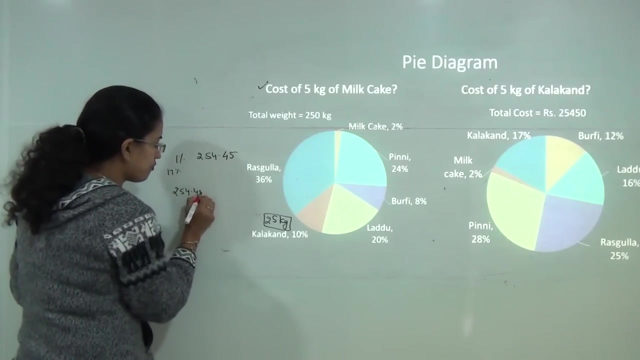 25 kg. and so what we will do is we will first find out for 25 kg how much is the cost, and then we will move around for 5 kg, what would be the cost? Now, as I said, 17% is Kalakan. now 1% would be 254.45, so 17% would be 254.45 into 17, and 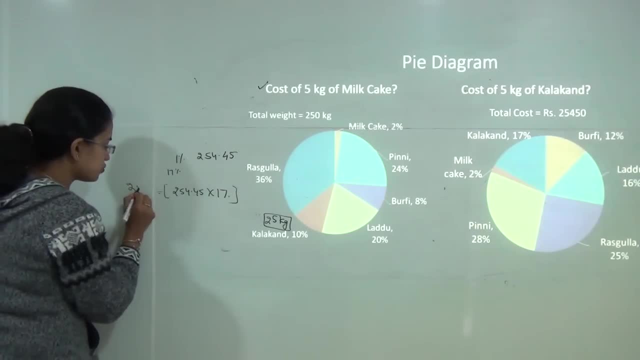 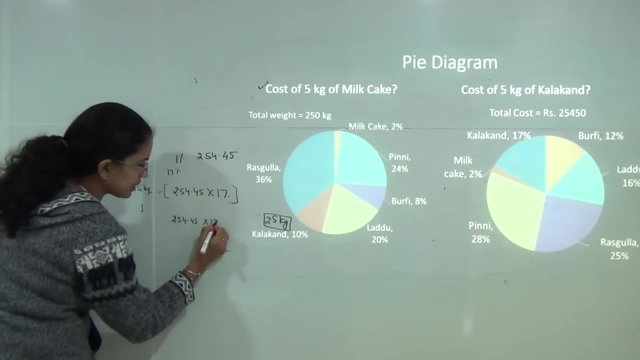 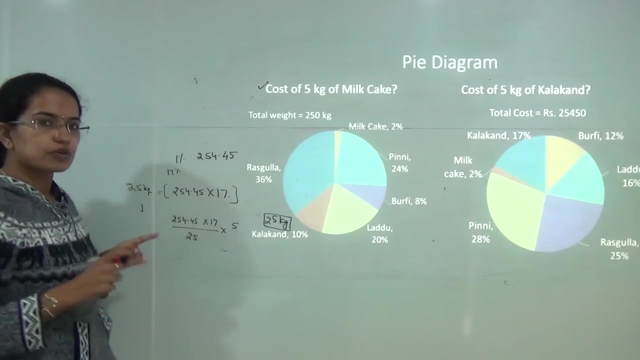 this makes up how much Kalakan. that is 25 kgs of Kalakan. So 1 kg would be 254.45 into 17 divided by 25, and 5 kgs would be into 5. now, as I said, if you keep the fractions as it is until end, it would be easier to solve rather than if.